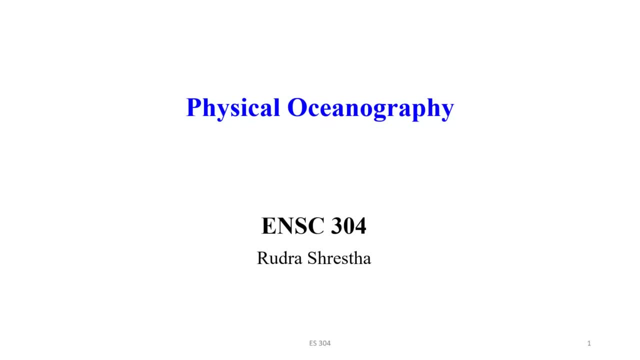 So now we begin the physical oceanography. So in this lecture we discuss the physical oceanography part. So in particular in this lecture we discuss the different variables, the pressure, temperature and the density, how they are different, how they vary in the ocean. 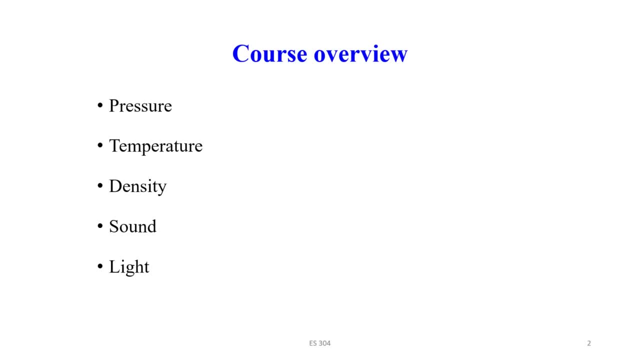 especially, and in the temporal mainly, how they are different in a different level of the different depth of the ocean. And we also discuss the sound and the light, how the sound travels in the ocean and also why we do, why we see the blue ocean. So that is. 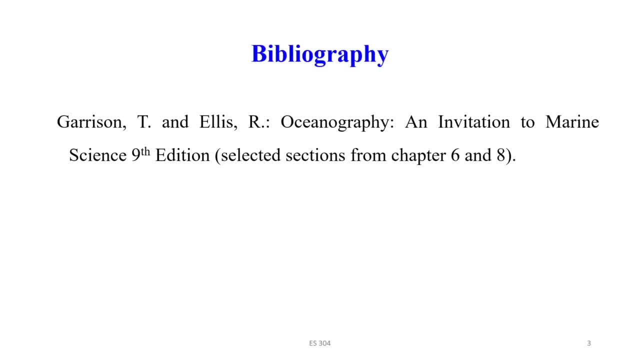 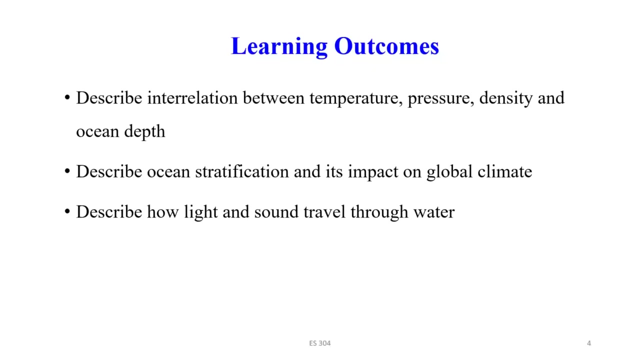 we are going to discuss in this lecture. So in this lecture it's mainly based on chapter six and chapter eight of our textbook, So it's not doesn't cover all two chapters but a selected section from those chapters. We will discuss inter relationship between temperature. 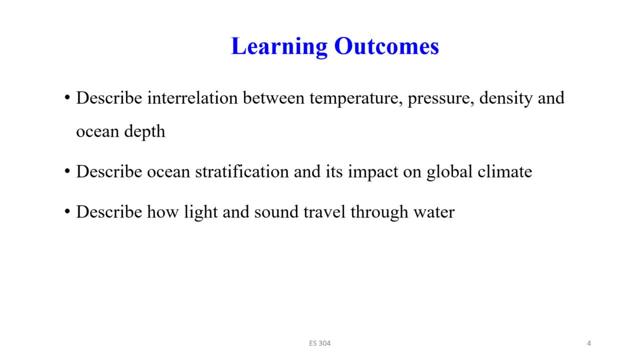 pressure, density and the- you know- depth of the ocean, And we also discuss different layers of ocean, the stratification and how does it impact on global climate. And also we'll discuss how the light and sound travel through the ocean and how can we use those signs to explore. you know. 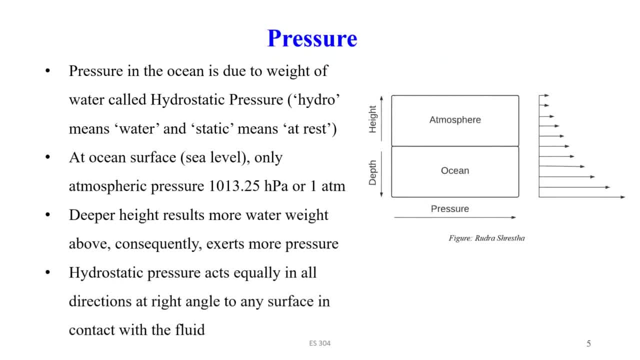 different scientific applications. Okay, Let's begin with the pressure in the ocean. you know that means it is a hydrostatic pressure. So the hydro means water and ecstatic means at rest. The hydrostatic pressure means it's a force per unit area and it's because of the weight of water. So let's look at the 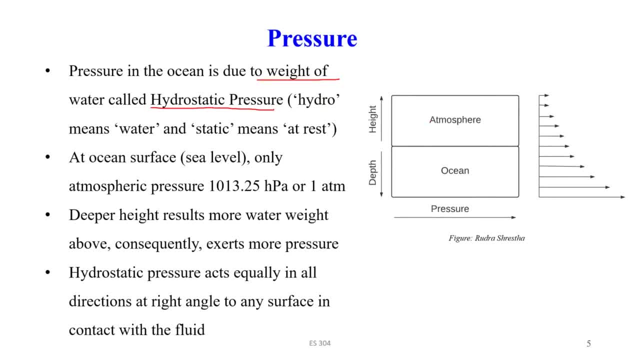 diagram. here on the right-hand side, We have an atmosphere and ocean and this is the, let's say it's a land, it's a surface and at this surface effect of the water, it's basically the hydrostatic pressure is zero, but we still have the. 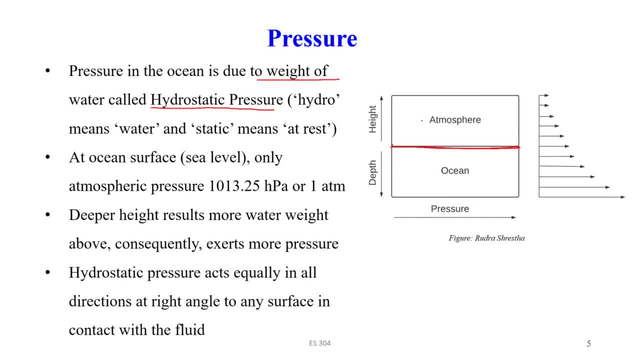 pressure from the atmosphere. So the atmosphere, it must say the pressure, we know this is the weight of air molecules above this, the surface, and that the pressure at sea level, the pressure of the atmosphere is 1013.25 hectopascal or is simply one atmospheric pressure. And when you go, 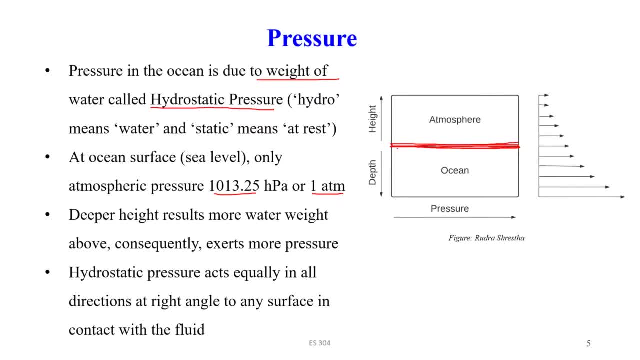 down the deeper so that you feel the pressure of the water. So let's say, this is the column of water and here the pressure of the hydrostatic pressure is zero, but when you go down you feel more pressure. okay, And that is because of you know the 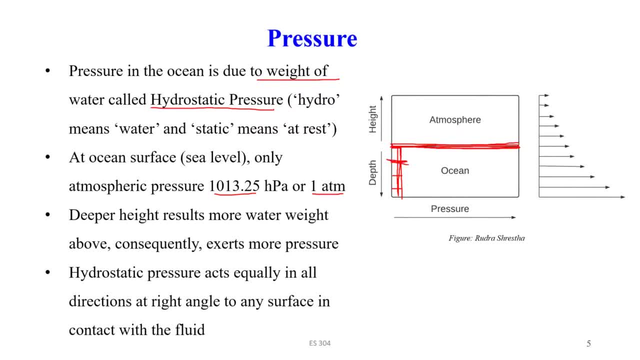 weight of the water. so let's say, at this level the pressure here is the water weight of the water you know. above this level, so this is, you know, this amount of water and when you go down, the water weight of the water increases and subsequently the pressure also increases. so we have the maximum pressure at the 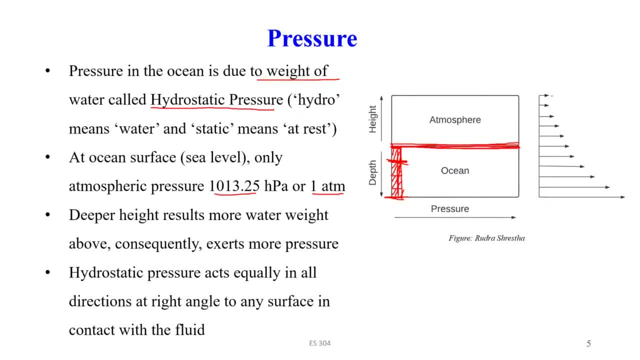 bottom of the ocean. and now here, this is the pressure diagram. so it says: in the bottom we have the maximum pressure here. so this is the magnitude of the pressure and it when you calculate pressure at any point here, you have to calculate the weight of this water plus weight of this. 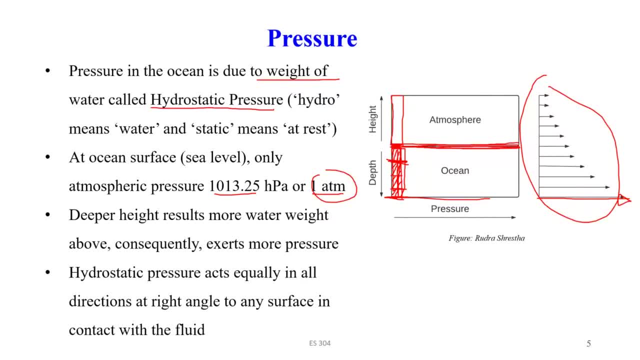 atmospheric column, which is the one atmosphere so here. so we have one atmospheric pressure and down here the total water pressure plus the air pressure- okay, so you have to consider that. and hydrostatic pressure X, equally in all direction. it right angle to any surface in contact with the fluid. so what does this mean? I 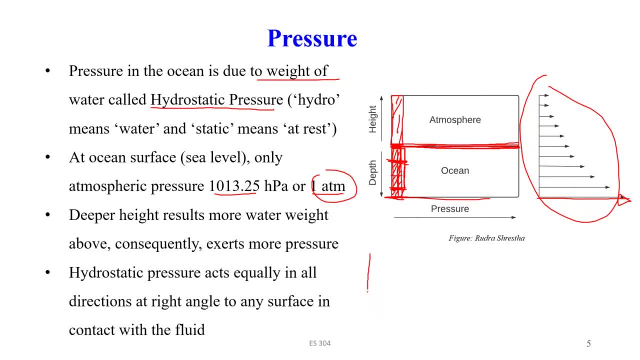 will explain this point with the help of the water tank. let's say this is a water upon to the atmosphere. so here and the water level is here. so I am going to draw a pressure diagram. so here side of the wall, so the pressure is like this. so because that means pressure, you know, increases linearly. so 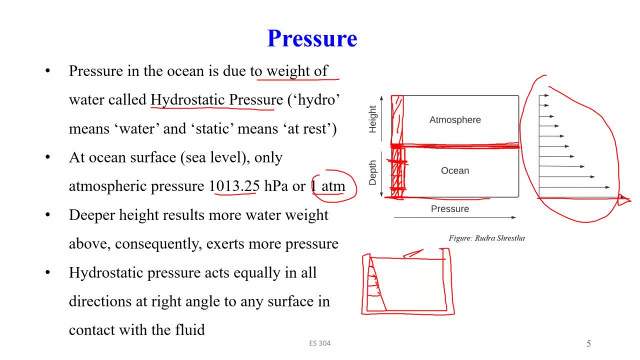 when you, you know, go more depth, so that means more pressure, because the water is, you know, uh, forcing this wall. you know, like, in the right angle, at right angle and also similar to this side, the pressure diagram is some something like this: okay, so this is the pressure diagram, and at the bottom, so, uh, you know. 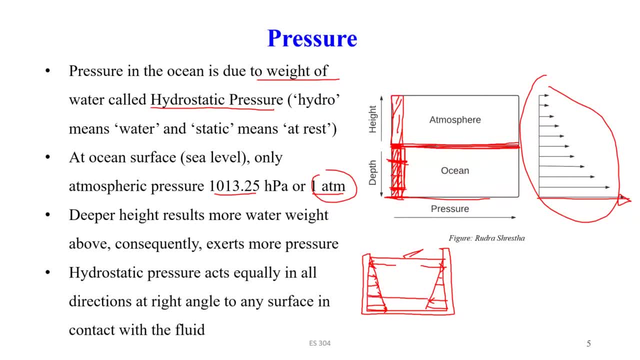 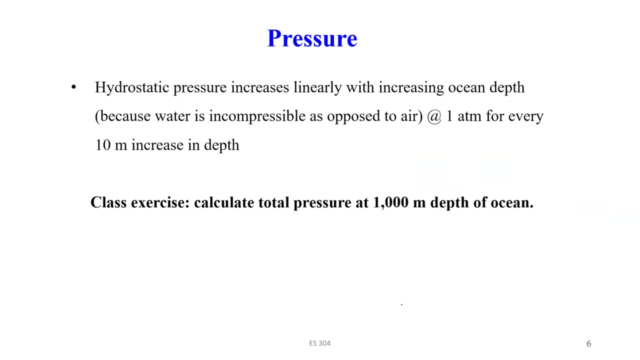 this is the amount of pressure. so here would be something like this. so this is the pressure at the bottom of the tank. so pressure: the water exert pressure equally in all direction and, it said earlier, hydrostatic pressure increases linearly with increasing in depth. The reason is the water is fairly incompressible, So you cannot compress water. 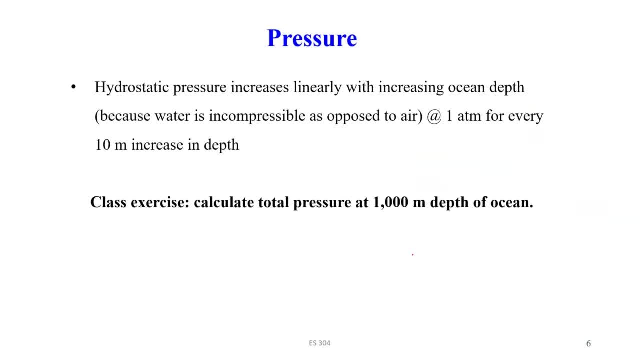 you know like we can do with the air molecules. So that's why you know it increases linearly. But if you remember the air pressure, you know it decreases rapidly closer to the surface of the earth and when you go up it decreases. you know different rate. So in the water, in the 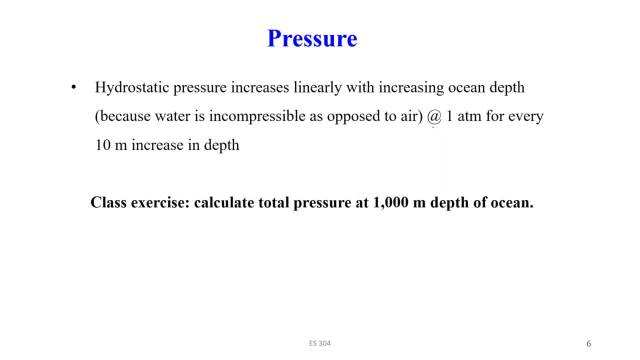 ocean. the increasing pressure is at the rate of one atmospheric pressure for every 10 minute. 10 meter increase in depth. So that means the 10 meter height of the water- ocean water is equal to the whole pressure of the atmosphere, pressure by the air molecules. okay, So I have one exercise. 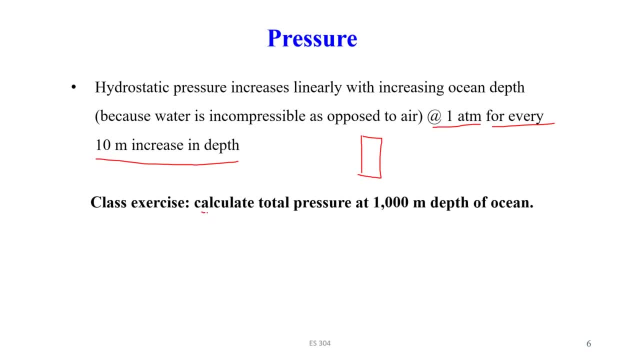 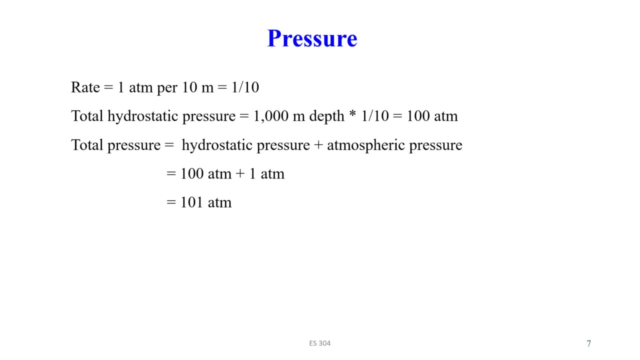 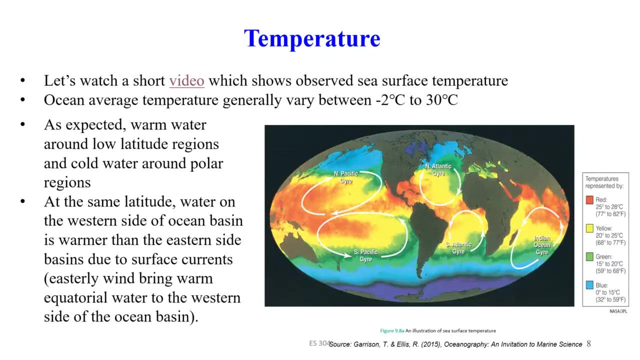 here for you. So can you calculate the total pressure at 1,000 meter depth of the ocean? So take maybe one or two minutes. The correct answer is 101 atmosphere, okay, Okay. So next one is the temperature. So I am going to begin with a short video here again. 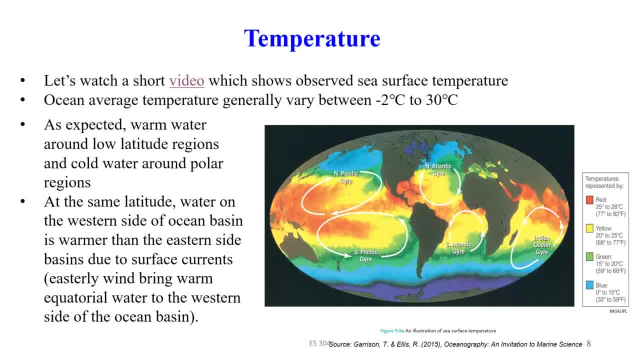 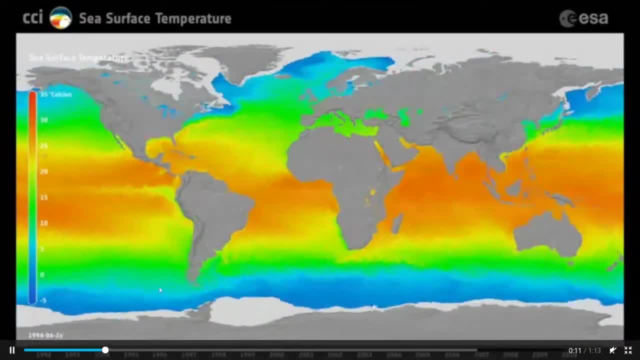 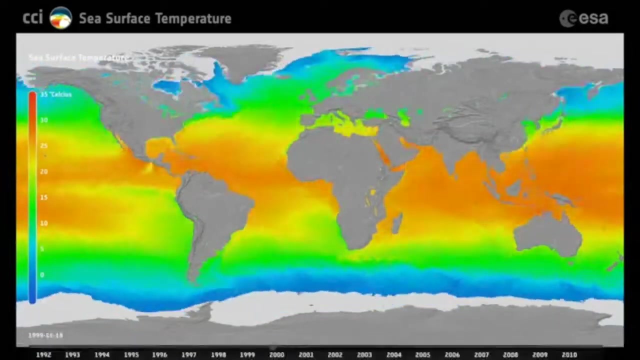 to explain the temperature of the ocean. This is the temperature animation from European Space Agency. So from 1992 to 2010.. Here we can clearly observe the seasonality. So this orange color is moving back and forth towards the northern hemisphere and southern hemisphere. 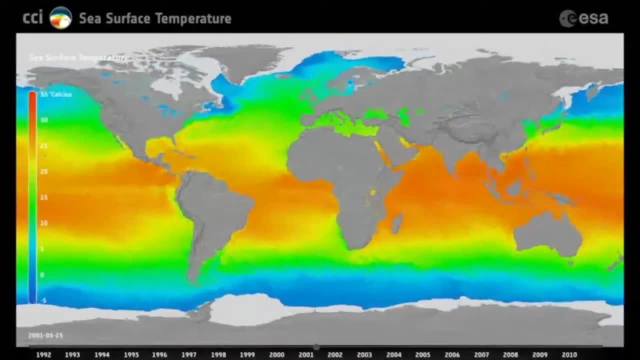 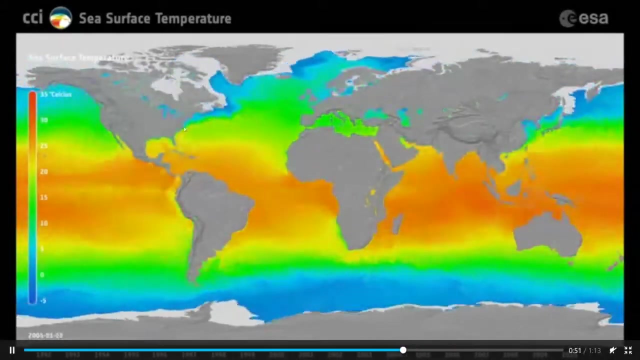 So this is, you know, it's something with the intertropical convergence zone, So it's kind of you know that they receive some maximum radiation, you know, during the summer season. That's why it's moving up north and south and we are also. we can see here I'm focusing on 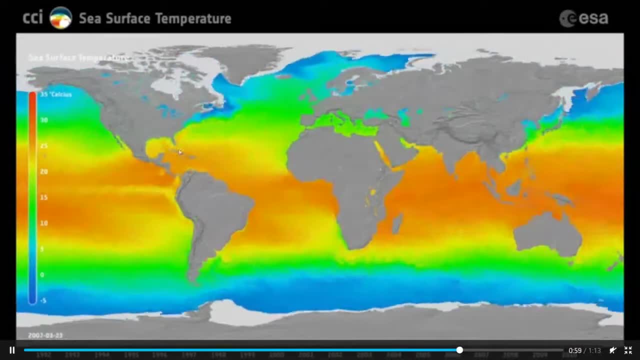 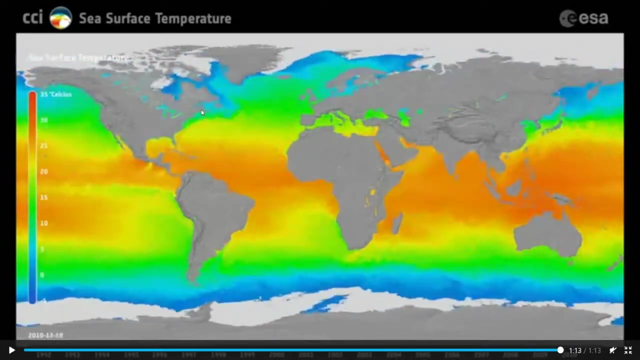 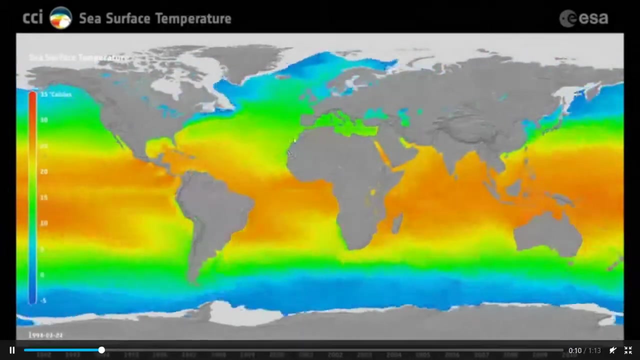 here Atlantic Ocean. so if you look at this part, so the east coast of the North America, so this part is, you know, like the warmer water is encroaching this part and and we can see this eastern part of the Atlantic Ocean, we still can see the colder, you know, water which is, you know, represented by the green color. 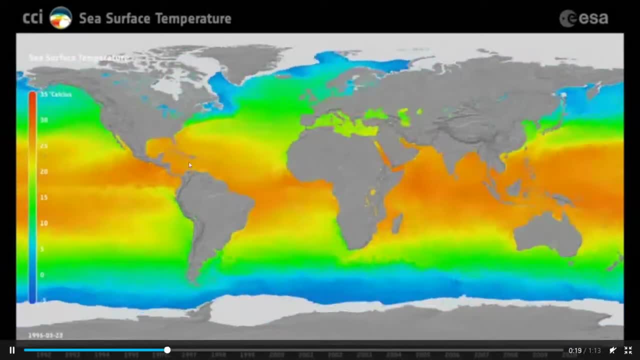 here so you can see the color bar and this part, the western part of the Atlantic Ocean. we can see the warm water and obviously the sea ice. it's going back and forth. this is because of the, you know, in the summer and winter, summer if you closely observe the month here. 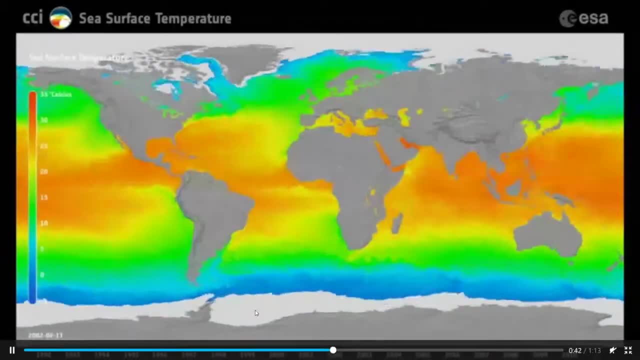 and summertime- this, you know, ice cover disappears and comebacks in the winter. same happens in the Arctic. so basically there are a couple of things we can make a note. so it's a the temperature of the ocean, you know, moving north out and the western part of. 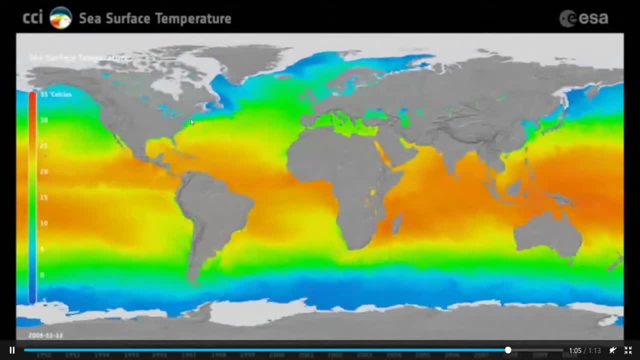 the ocean body. you know, warming, much more warming there, and eastern part is still. we can see the colder water, especially the boundary between land and the ocean, and the seasonality of, you know, the ice. you know something: summer it disappears and come back in the winter. okay, so is we. 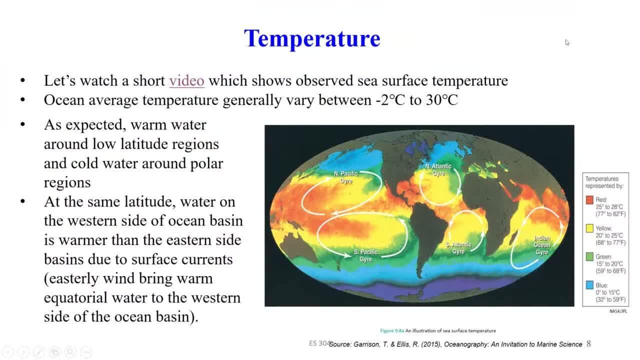 on that animation. the ocean temperature, you know the between minus two degrees Celsius to 30 degrees Celsius and it's expected the warmer water around the equatorial region, in the colder water around the polar region, that's the sun also, um, we observe at the same latitude water on the western side of the ocean, you know warmer. 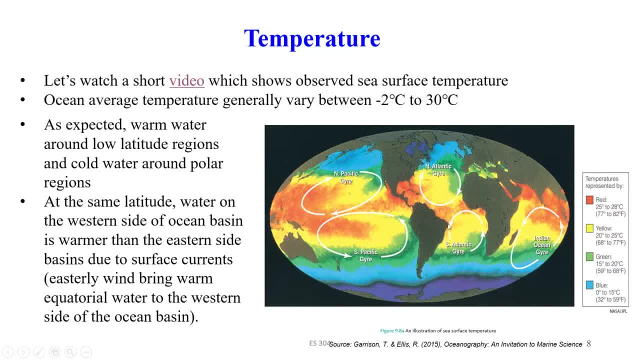 than eastern side, and even more clearly we can see here equatorial part, the low latitude region in the both southern and northern hemisphere is, you know, the color red color, which is, you know, the warm water temperature, and also we can see here this part, the Atlantic. 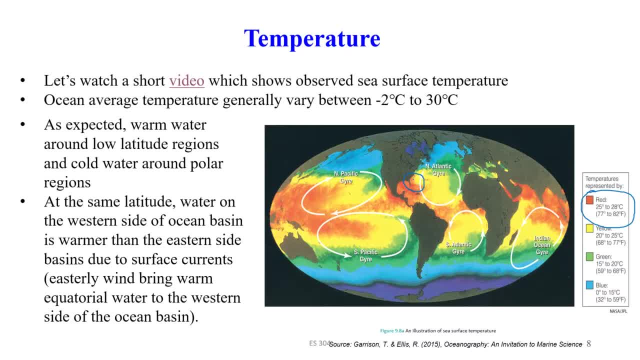 Ocean, the western part of the Atlantic Ocean, you know, it's warmer than the eastern part of the ocean, and the same thing here, Pacific. here it's a colder water and it's not, but this part is, you know, warmer than the eastern part of the ocean and the same thing here. 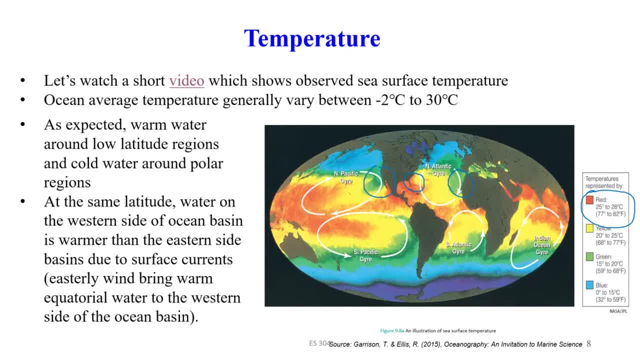 you know it's warmer, okay, and the reason for that is it's a circulation, the wind circulation. so we have to remember here, you know, trade wind, easterly trade wind and westerly wind, polar easterly. so let's draw roughly the line, the latitude line, here. 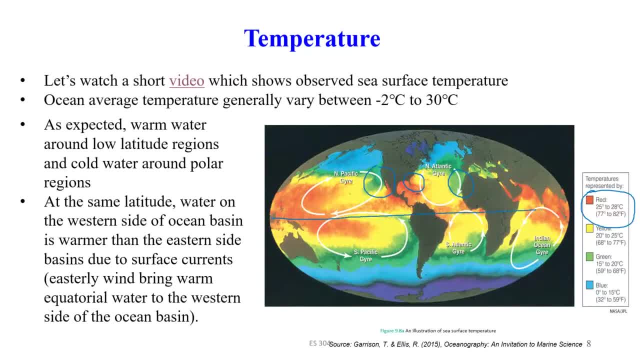 so here it's around the zero degree equator. it's not perfect, but let's just, you know like, make a rough draw, a rough line here and around the 30, so it's somewhere here, hopefully, and the 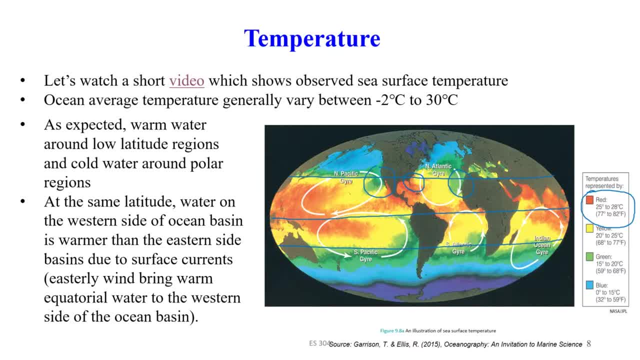 southern hemisphere it's something like this. so here these parts we have, you know, easterly wind, so that's blowing from east to west, and understand this phenomenon we talked about previously. see, really important here too. 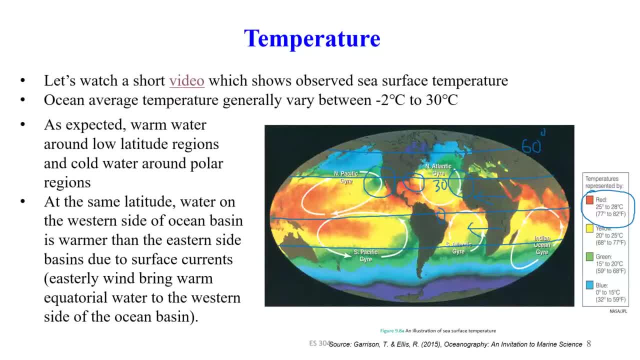 so we have a betray prat now. if weановy of the ocean, the windлю, and we have a westerly wind, so one for western part of us. it's another fleece part. we have joined in with other parts of the ocean around them, so it's transfers away slightly in that direction. okay So, and disappeared, Okay So. and we remember here that this is, this is. you know, we remember that. you know this is dry air give to the south, or these are for migration, but we know that technology creates. 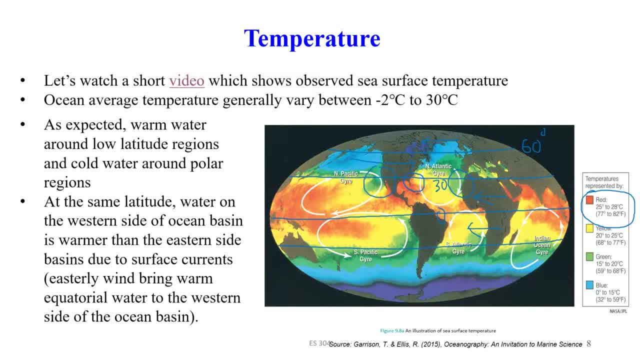 of the ocean and cold water in the eastern part of the ocean. uh, here this easterly the trade wind, you know, blows the surface water in this direction, the, you know, from east to west direction. when that water current hits the land, the continent, it, you know, deflect that way. so it has two effects. one: 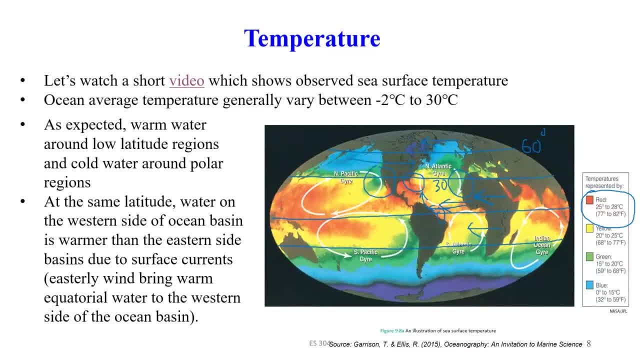 is because of you know, it hits, it encounters the continent, and the other one is the coriolis effect. so that way in the northern hemisphere that deflect towards the right and in the southern hemisphere deflects toward the left. and what? the water in the equatorial region? 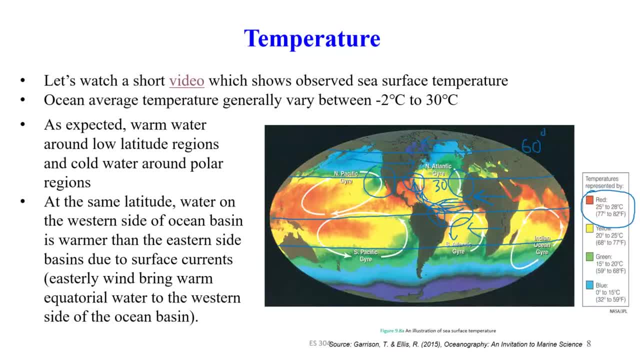 it's a pretty warm and that travels towards this direction. so this, the western boundary, uh, is, you know it's the warmer water and, on the other hand, this westerly wind, that is, you know, 30 to um 60 degree latitude, which is, you know, pretty cold as compared. 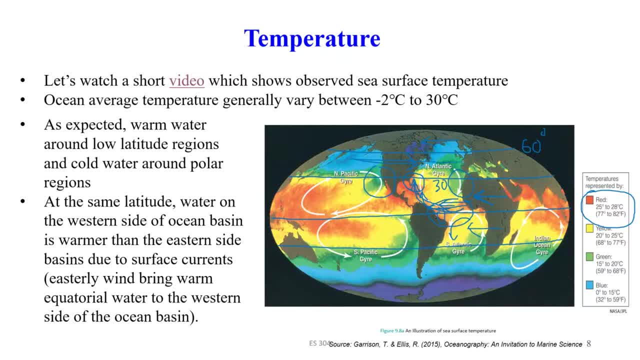 to the equatorial water that blows the water current towards this direction and deflected by a coriolis force, and also uh, due to the encounter with the, uh, the continent, so that is the cold water you know, encroach this part of eastern part of the, you know ocean. so and 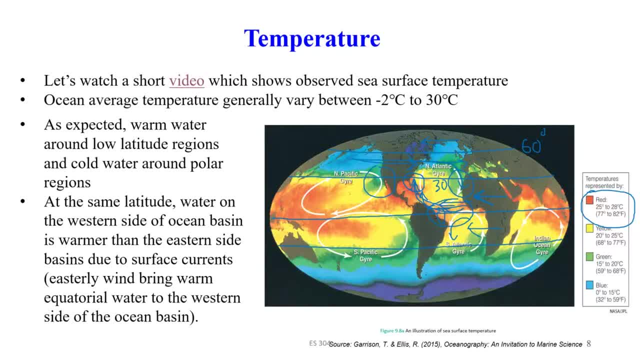 that make a kind of, you know, a circle, and this um is called western boundary and this is called eastern boundary. we'll discuss more about the circulation in the coming weeks, but uh, you know, this is just to give you some idea, and this is called the zire, so this circulation is called. 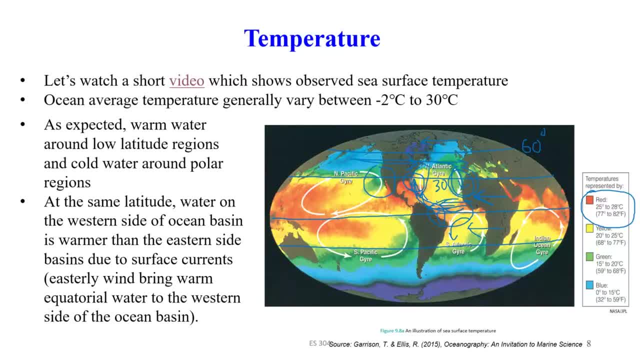 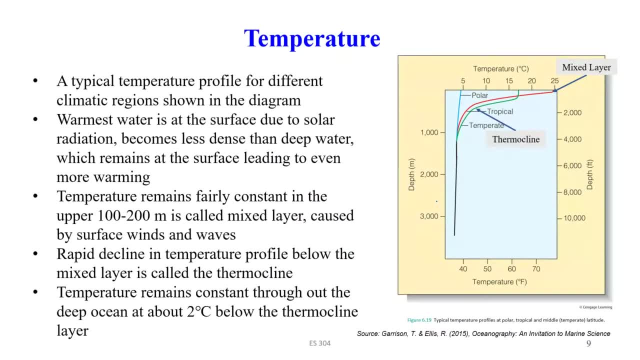 zire. so we have couple you know um you know theoration of the Racoon region or lake STAR, yourself know you have your come here, your, you know several. and now let's uh have a look on the temperature profile and this, this figure on the right hand side shows um the typical uh temperature profile. 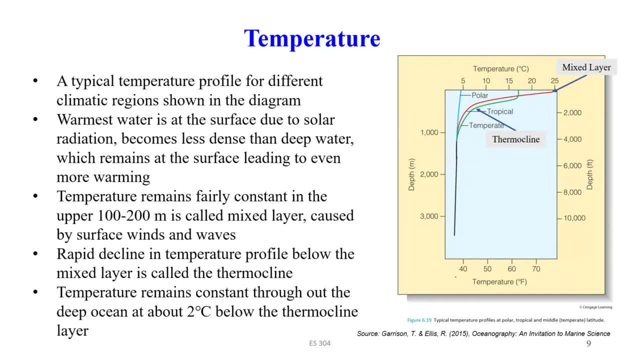 of the ocean. So here the x-axis is temperature and y-axis is the depth, And here the red line represents the tropical- you know the temperature profile in the tropical region- and this green line is the temperate region and this blue line for polar region. As expected, the tropical ocean has, you know, warmer water at 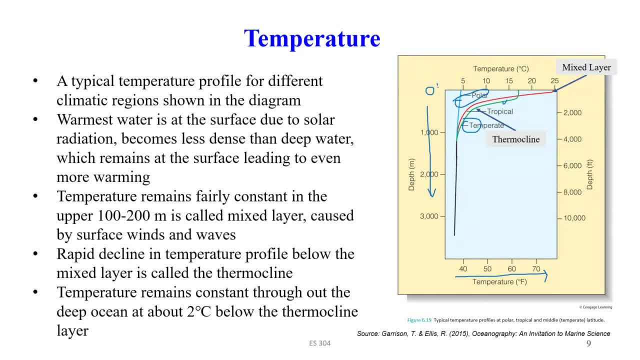 the surface. so the surface, the zero meter depth, and it, you know this layer is called the surface layer layer because this is mainly affected by the, you know, warm, by the solar radiation, And it remains, because it becomes less dense and, you know, it stays on the surface layer. 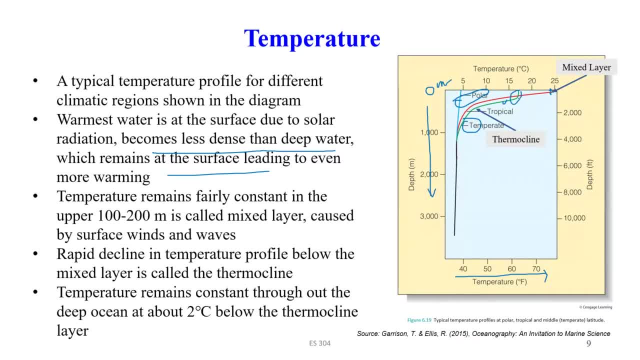 of the ocean And this is similar to, you know, temperate region and but we can see the impact. you know it's less here in the polar region because polar region gets less solar radiation And this surface layer is, you know, normally 100 to 200 meter depth. 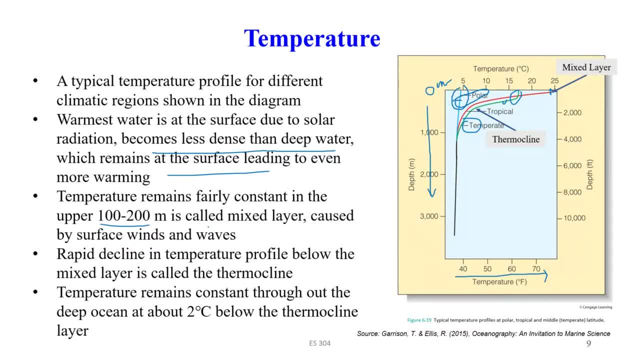 It's mainly caused by, you know, mixing of, you know, the radiation, the energy, because of the winds and the waves And after that, Okay, So after the mixed layer, or surface layer, the temperature decreases rapidly with height and that the layers. so you can clearly observe here, you know, in the region, so it's a. 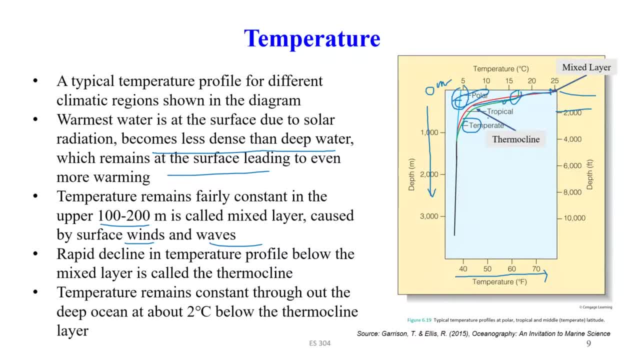 you know very short layer. the temperature decreases, you know very rapidly, from you know around 25 to you know Fahrenheit to you know like 45, so it's a pretty. you know rapid reduction or decreasing of the temperature. 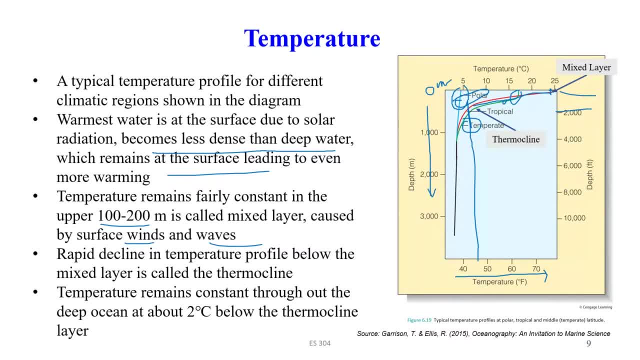 So that also happens in the temperate region. So here the green light, so it's, you can see here. but this effect is less significant in the polar region. So that layer is called thermocline layer, where temperature decreases rapidly with. 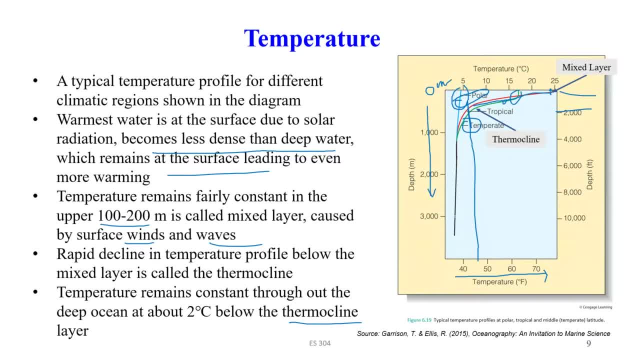 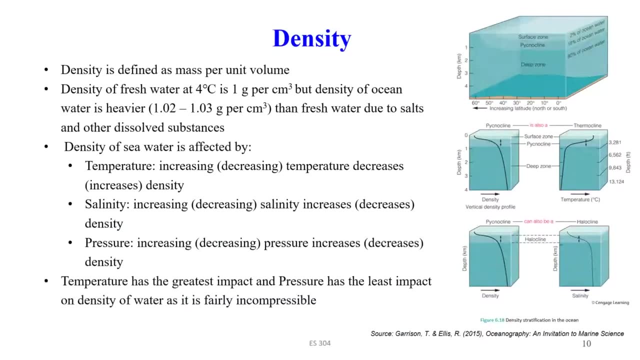 height, Okay. And below that layer, below the thermocline layer, temperature decreases rapidly with height, Okay. So the temperature remains reasonably constant and it's about two degree Celsius. So next one is the density. So density, as we discussed in our atmospheric part, it's a mass per unit volume. 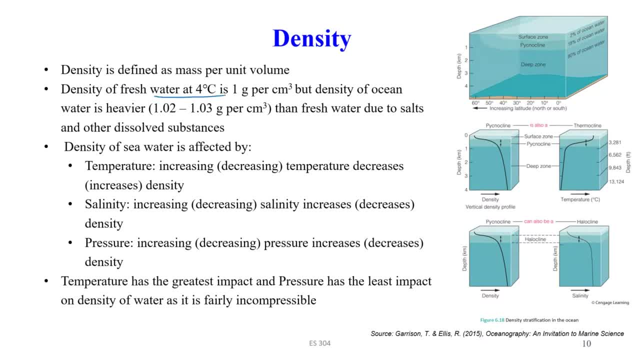 And density of fresh water at four degrees Celsius is one gram per meter per centimeter. So at four degrees Celsius density of water is a maximum. so you may be aware of this. If not, let me draw a diagram that explains U. So here it's a temperature in the x-axis. 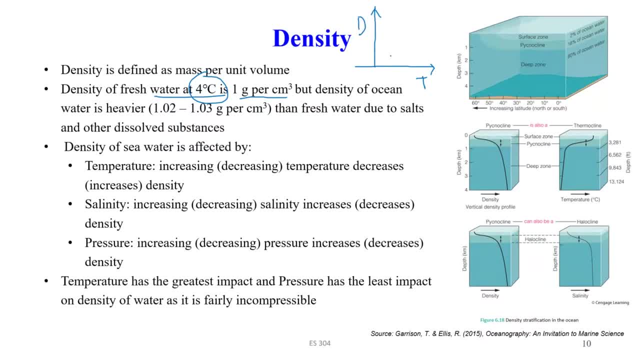 and density in the y-axis: Okay, Okay, So the density curve looks like this: The density, this is the density curve, Okay, And this maximum is at four degrees Celsius. So maximum you know here at this point, so one gram per centimeter cube. 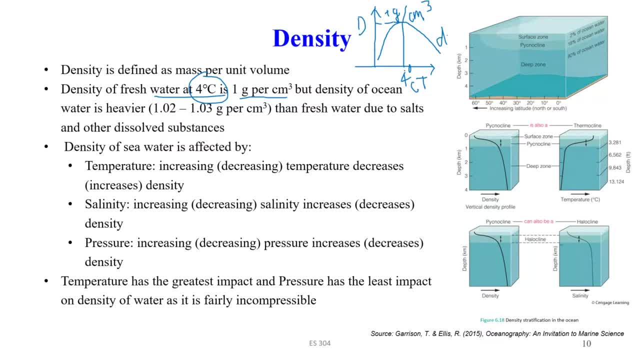 So it's a maximum density of water at four degrees Celsius. So when you decrease a temperature below four degrees Celsius, it's a mass below four degrees Celsius. the temp, you know density is gonna, you know, change and you know. 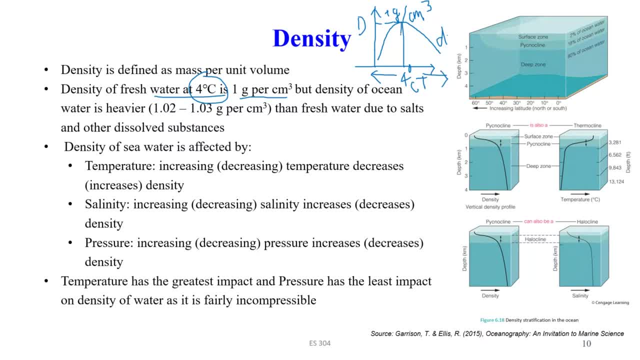 in both directions. Maximum density is heavier. So water is, you know, heavier at four degrees Celsius. So in. but in the case of the ocean water, it, you know the density, it's slightly heavier than the freshwater. So it's it's about 1.02 to 1.03 gram per centimeter cube. It's because 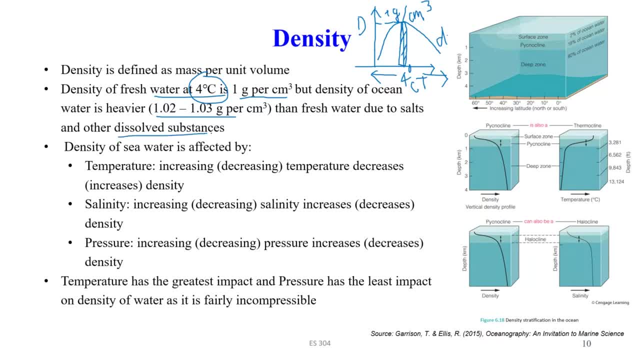 of the dissolved salt. There are so many dissolved substances in the ocean that makes ocean water heavier And the mainly the density is affected by the ocean density. Ocean water density is affected by the water density. That's the main problem of the ocean water density And it's 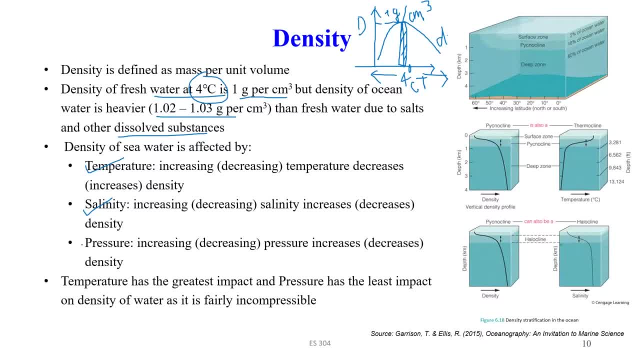 you know it's, it's, probably it's the main problem of the ocean water density. It's the affected by the temperature, the salinity and the pressure. So increasing temperature decreases the density. and this is true for you know, like here. 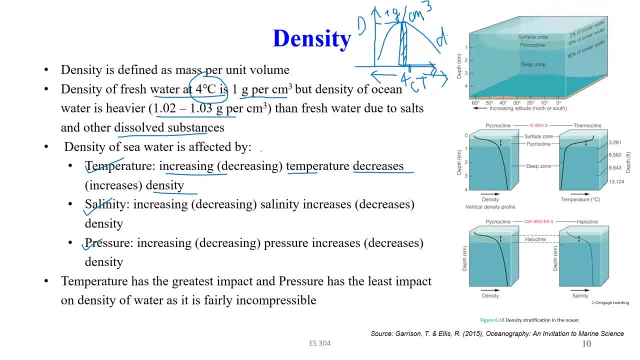 so above the 4 degrees Celsius And you know below, then you might wonder why. you know, like, if we decrease the temperature below 4 degrees, and then what is causing? you know the decreasing density, Because when the water is closer to 0 degrees Celsius, its structure it makes a cluster. 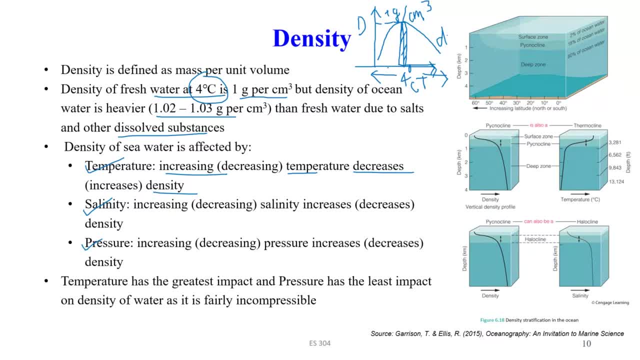 of the structure which is, you know, similar to ice. So, and that ice shape is what we call ice lattice shape, and that is, you know, like a different shape, something like this. So, if you Google ice lattice shape, so, and that makes the shape something like this: 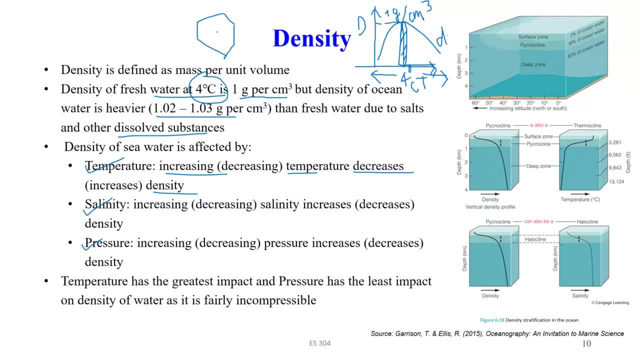 And it creates the void and you know it becomes the less dense. So even still the water is liquid, you know, at 0 degrees to 4 degrees Celsius, but its behavior decreases So it makes the cluster of, you know, the structure like ice lattice. 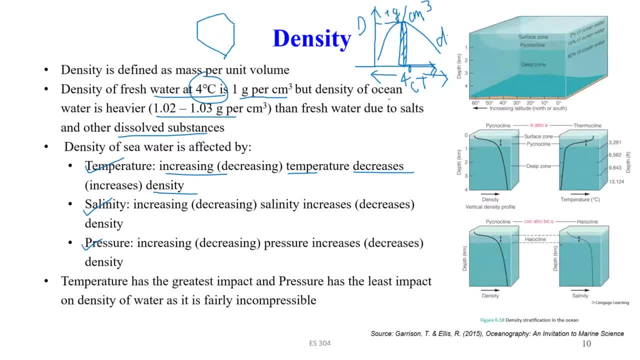 That's why its density decreases when we, you know, reduce the temperature below 4 degrees Celsius And above 4 degrees Celsius when we have, you know, the more energy, the water molecules more faster and that we make the water molecule less dense. 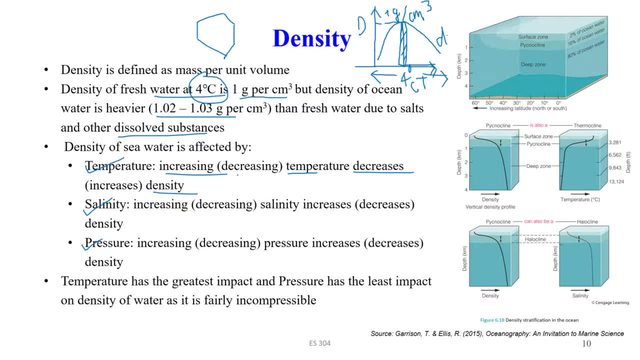 Okay. And likewise, decreasing temperature increases the density And salinity. increasing salinity increases, you know, the density, and vice versa. Decreasing salinity decreases the density. Okay, The pressure. Increasing pressure increases density, And vice versa. 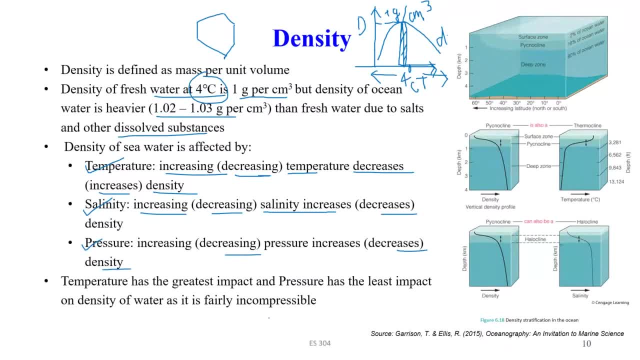 density and the decreasing pressure decreases density, but the temperature effect is quite significant and we can clearly see here. so here is the depth and the density in. you know, increasing this direction and the effect of temperature is, you know, like just the opposite way, as we discussed earlier. so increasing temperature means, you know, sorry, decrease pressure means. 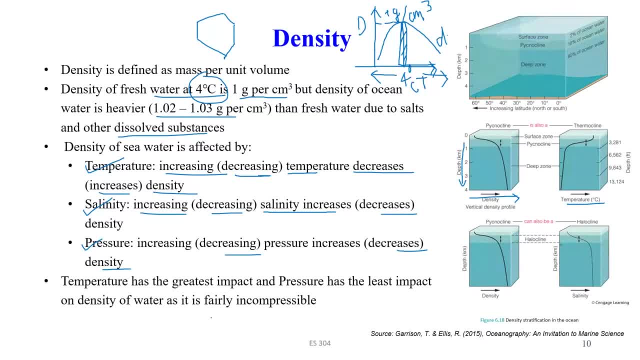 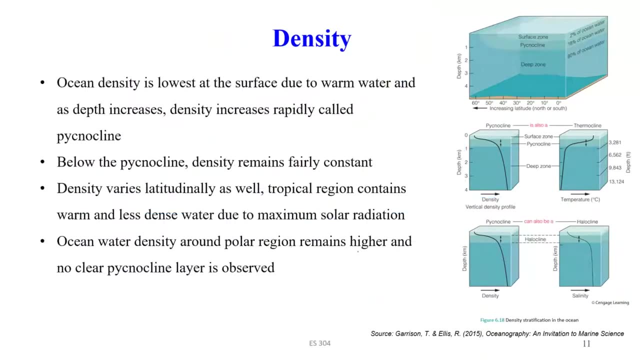 the increasing the density. okay, and pressure has the least impact on density because it's a, it's a fairly incompressible: you cannot compress the water. so density is a lowest in the- you know- surface layer because the surface layer, you know, is warm because of the radiation and 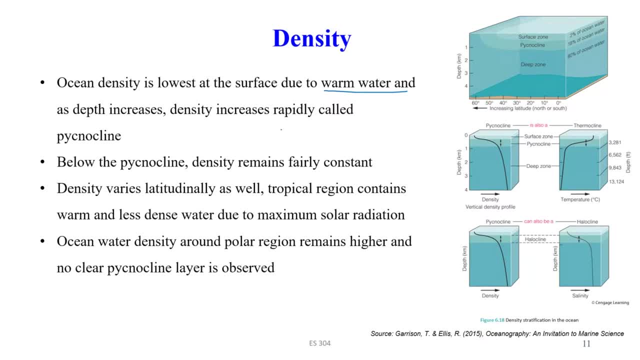 decreases rapidly and it over. you know, like, when we go deeper, when we increase the depth, density increases rapidly and that is called the peak. no climb. so here this layer, so, uh, when, um over, you know, when we move uh, uh, downward, then density increases. you know this, uh increases rapidly and this is um the effect, as we discussed earlier the effect. 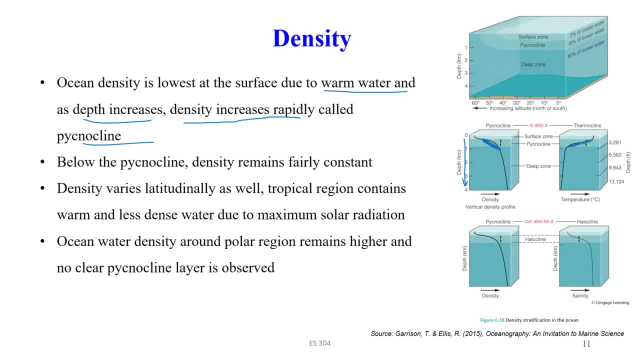 of temperature is quite significant. so it's you know, temperature in temperature uh decreases uh rapidly here the thermocline layer, and uh density increases here. so this layer is called the peak nook line, and below this level density remains fairly constant. here so the deep layer. 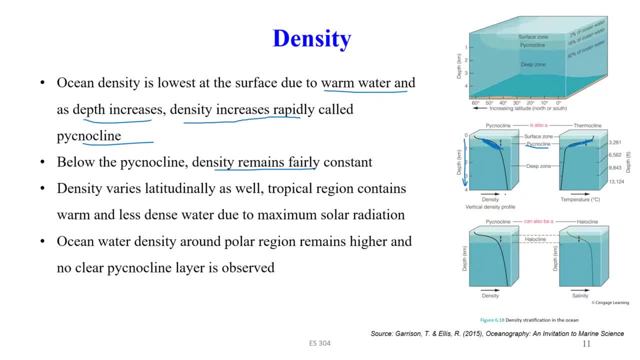 and the density also. you know like different. we can observe different density not only in the vertical layer but also the horizontal direction at different latitude. so tropical region, it you know like it receives intense solar radiation and that makes the water molecules warmer and less dense. but when we move to the polar region, you know that ocean water becomes. 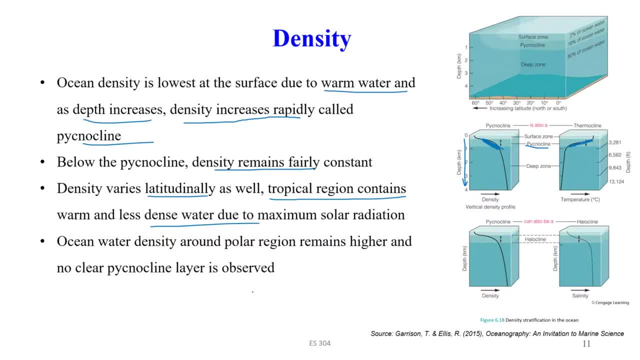 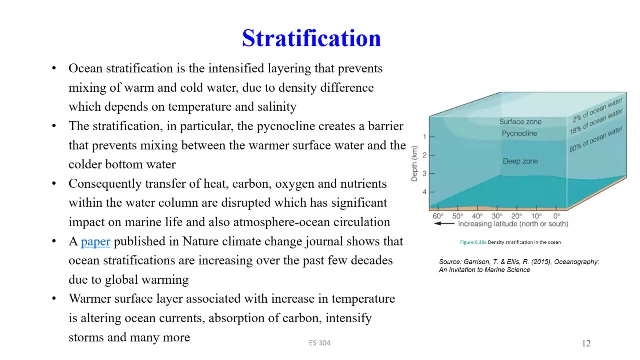 you know, more dense due to the less radiation and we don't clearly observe the pycnocline layer in the ocean and we don't clearly observe the peak nook line layer in the ocean. i mean in the polar region. stratification is um, a layer in the ocean, um in the ocean. so basically, 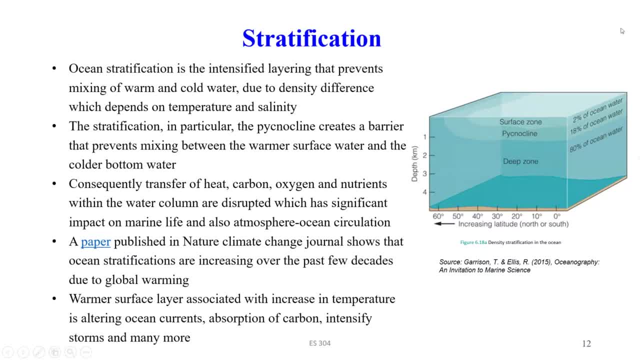 we have three different layers. we have a surface layer or surface zone, the pycnocline and the deep zone, and they are mainly due to the density difference and again, the density depends on temperature and salinity, and they, you know, then, that layer, that stratification, is you. 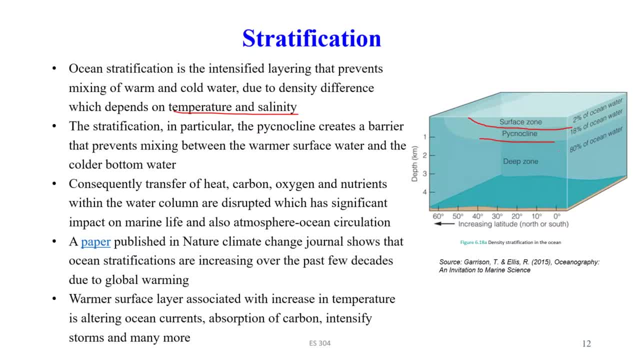 know uh, preventing the different um, the water in water, from different layers, to mixing up, and especially that this pycnocline layer, which is a sharp you know, decrease um, increase in density. you know uh, it's going uh when we go uh downward, the when you moved um down, so it's a sharp. 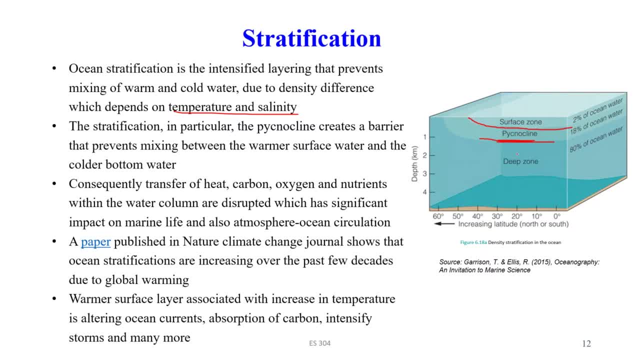 increase in density. so that is uh particularly uh preventing uh the mixing between uh the water from deep region to the surface surface layer and when we have that situation, um, it has a very, you know, important in terms of heat transfer. so the surface layer they, you know, absorb heat from the sun and 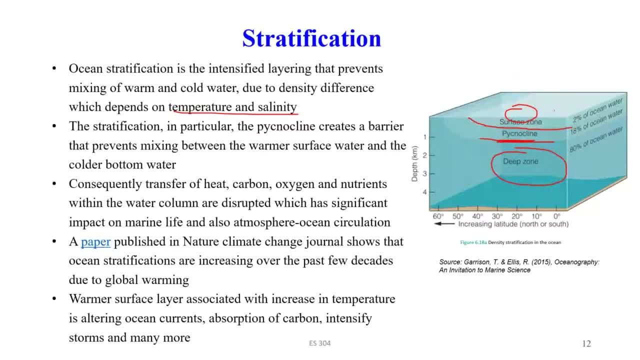 without transferring to the deep layer, it becomes very hot and hot. and also the oxygen where you know the marine life needs: the oxygen that cannot transfer to the- you know- deep layer and the nutrients they you know like it cannot come, because cold water contains lots of the nutrients that cannot transfer to the surface layer, so it's a 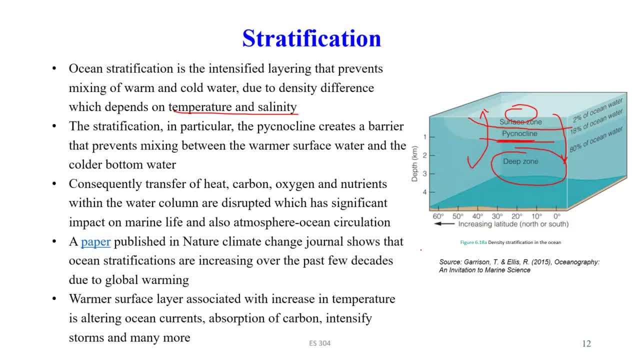 it has a complex, you know, interactions between the surface layer and the deep layer. when that doesn't happen, that system just stop working. and recently there is a paper published in a nature climate change journal. so this is one of the very high index journal. that means when you publish something in this journal, that means that's quite 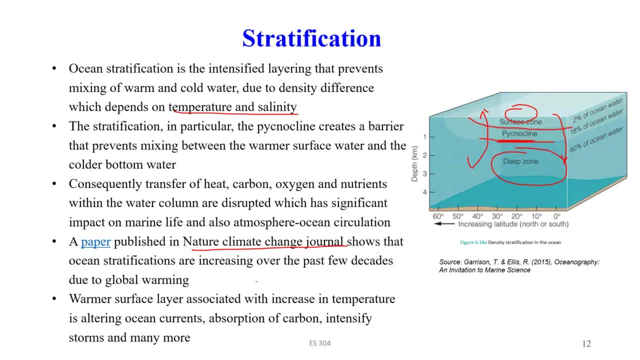 significant, so it does. pop paper here now shows that the strategy, the ocean stratifications, you know are becoming stronger in, particularly over the past few decades, and that you know that also this they said this is related to the global warming. so the global warming, you know, they increase the surface. 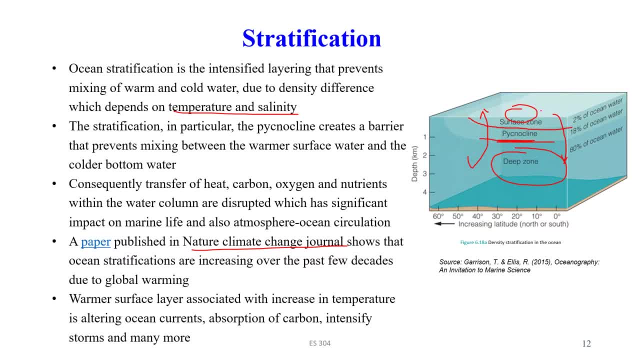 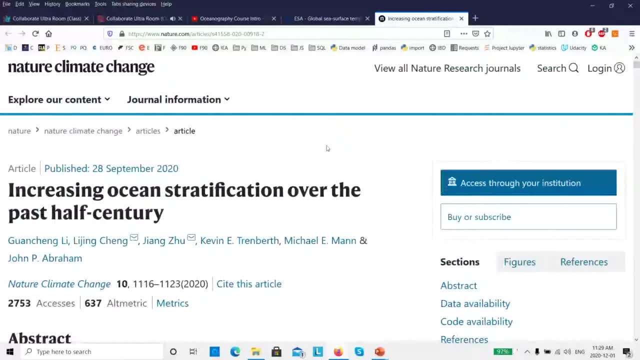 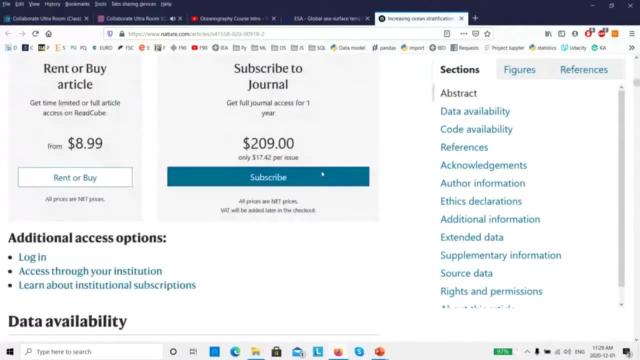 temperature and becomes the water- they are less dense and big, you know- and becomes more stable. so you can download. it's a free, freely available, it's open access. you can download and i think so i downloaded last time. it says something here. it's showing them price. 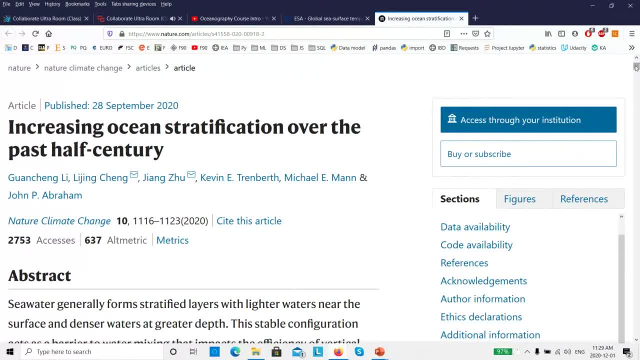 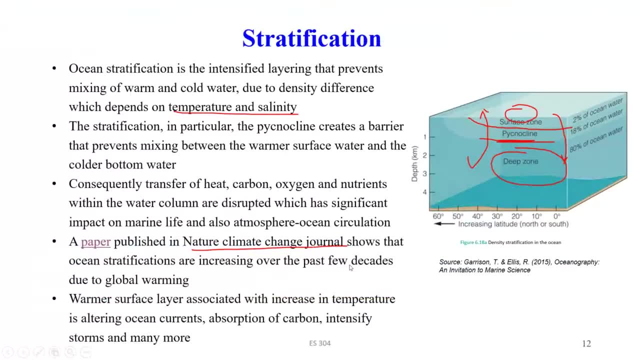 anyway. so if not, i would probably upload in the moodle i last time i downloaded. so basically, um the the article, uh the paper, um indicating global warming. it's uh, you know, uh impacting this, uh study stratification. it is been going on for several years and the research shows that city, rather than just global warming. 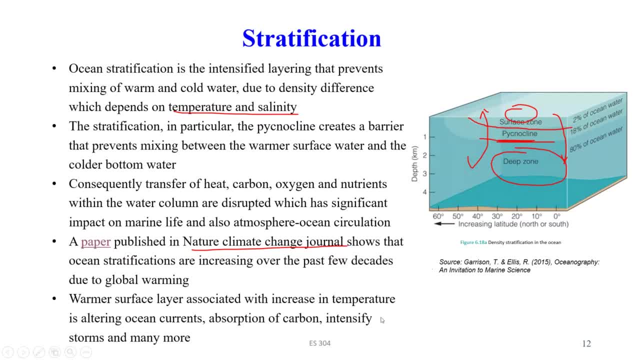 will uh be increasing during all of these information acts and also in the hydrocephalic pick winners. it is already now thousands of five hundred thousand anderer, this kind of same myself employee. so it will be uh very, very, very, very stren adjourned. but, as you know, 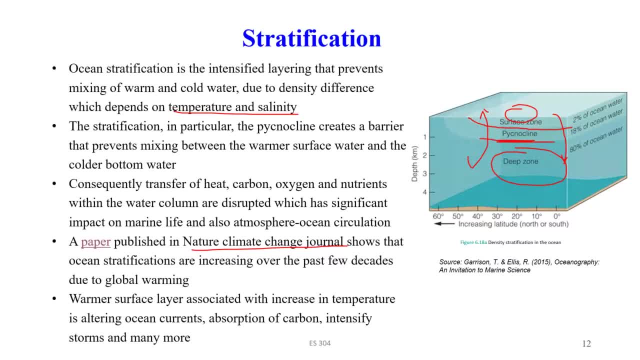 during the global warmingли. it has developed somehow to the goal to have deeperchu uh specific Now you protest- meet its nature: climate change. there is one interesting case. the other one is the earth that i mentioned, actually four or five bosna city impacts, uhger who have become stronger and when we have this strong stations and uh that modify the ocean currents because the surface of the ocean becomes warmer and warmer and that definitely changes the surface currents and also absorption of you know, differentοι. 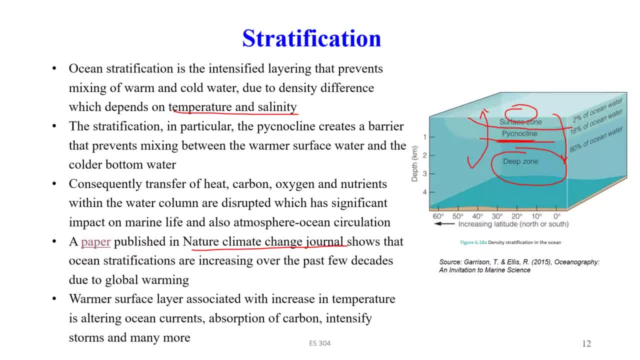 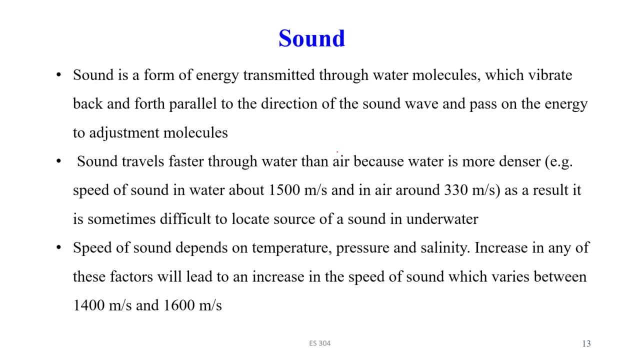 the carbon dioxide or oxygen, and intensify the storms, let's say hurricanes, and there are many more, you know, factors affected by this strong stratification. sound is a type of energy and that energy is transmitted through the water molecules, you know, and it vibrates, the water. 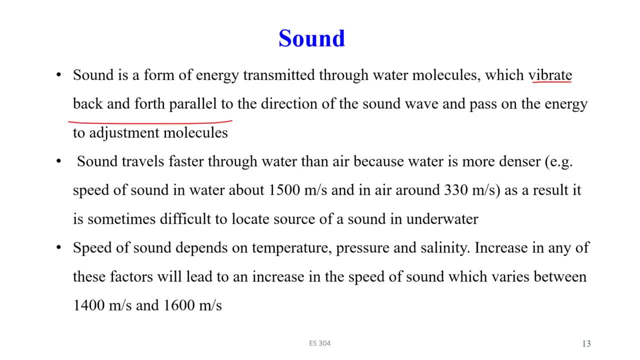 molecules vibrates back and forth to the direction of the sound traveling and pass that energy from one molecules to the molecule next to them. okay, and sound travels faster. inter is compared to air so, which is actually much faster. in water it's around 1500 meter per second, but in air sound can sound only travels around 330 meter per second. so 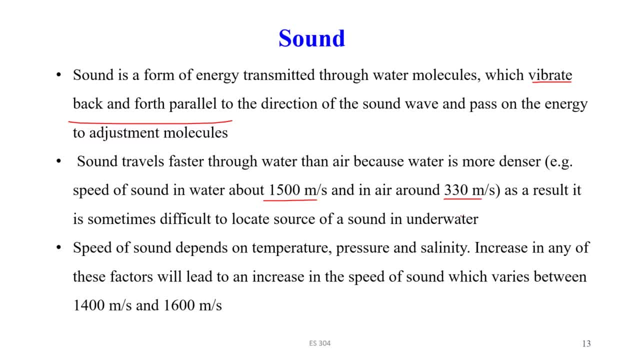 it's about almost five times, you know, faster, uh, in the water, and some, you know, sometimes it has, uh, you know like, different consequences in terms, especially in terms of finding, um, the source of the sound, because it's a, you know, too fast and our ear, ears cannot, you know. 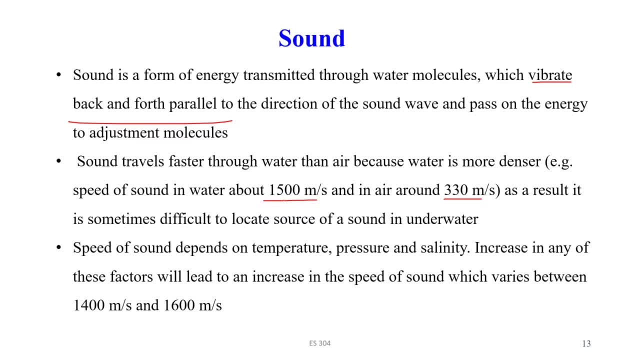 different. they are, you know, arriving in our eardrums in exactly the same time. so, uh, i mean very, very, very small, um, you know, difference in time. so we it's hard for us to differentiate which, from which direction, the sound is, you know, coming from. 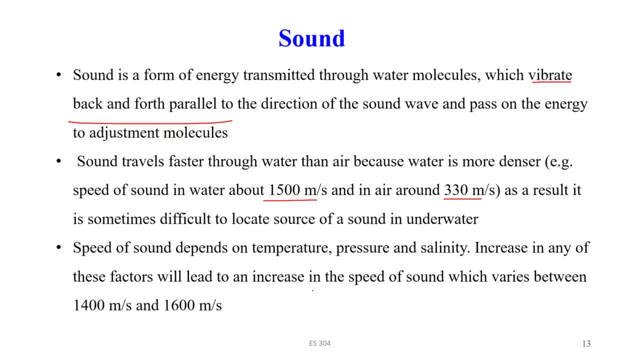 and the sound um. the speed of sound depends on the temperature of ocean, the pressure and also the salinity. so increase of any of these variables um increase the speed of sound. so mainly in you know that lies between 1400 meter per second to 1600 meter per second. 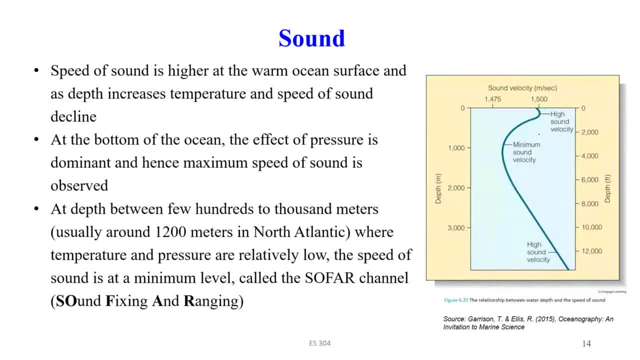 so let's look at uh the diagram here um that. this diagram shows the you know the different velocity based on, uh the depth of the ocean. so uh here um the depth increasing on the surface layer- here zero meter- and the velocity of sound in the x direction. 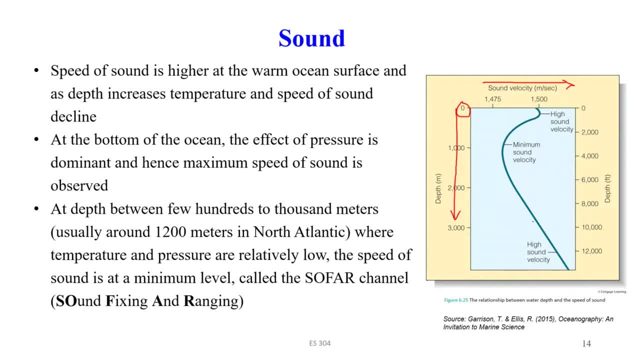 and this the line, this the solid line shows um, this speed of the sound at different altitudes. so here were the at the, um the surface layer. so where um the temperature is, you know, maximum, it increase the speed of sound because, um, the speed of sound is affected by temperature, the pressure and the salinity. so here, 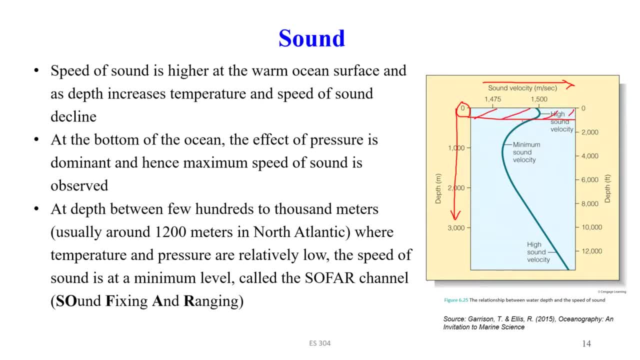 the surface layer we have a maximum temperature, we observe the maximum speed of the sound. so when we go deeper um, the temperature decreases and but gradually pressure increases. so here, let's say from here the bottom, the deep layer, we have the less temperature but we have maximum uh this, uh the pressure. so that's why we are, we have um the speed of sound maximum in this. 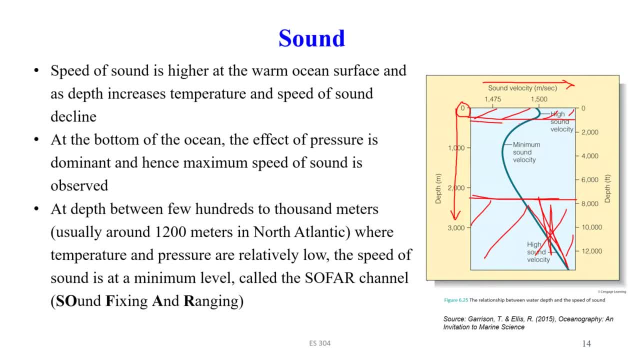 uh in this part, okay, but in the middle we have the minimum uh sound velocity, uh, where um the temperature is, uh, reasonably, you know, uh lower and the pressure also, uh the lower at this this layer. but this uh, this layer, um, in terms of the north atlantic, is around 1200. 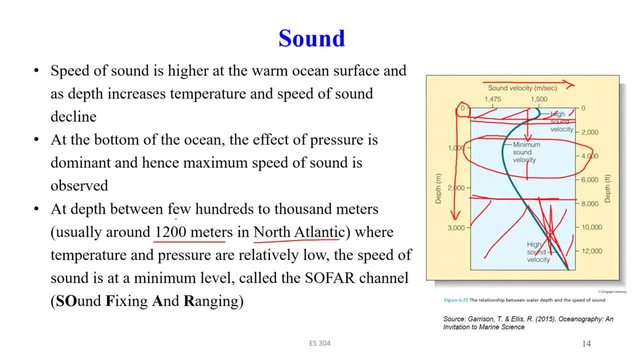 in general, this layer lies, you know, between few hundred meters to the thousand meters and this layer is called the so far layer or so far channel, which stands for sound fixing and ranging. so this layer is called sound fixing and arranging, okay, the so far channel. and in this layer the speed of uh sound is at minimum level, at lowest level. 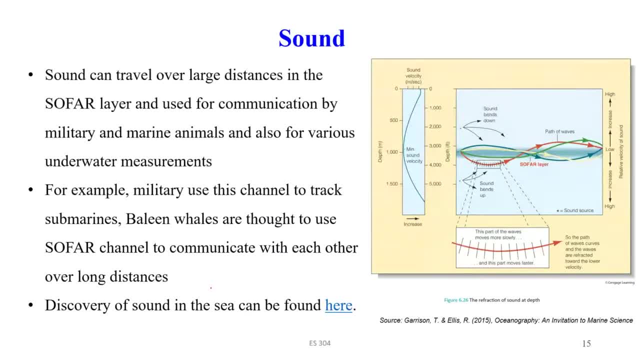 but it has, um, very, you know, um important practical uh applications, um, so, um, then, the sound in this, um, the so far channel, the so far layer, can travel long distance and that is used by military uh, for, you know, to track the submarines. and also this layer is used by, um, the marine animals, uh, let's say the whales, the, 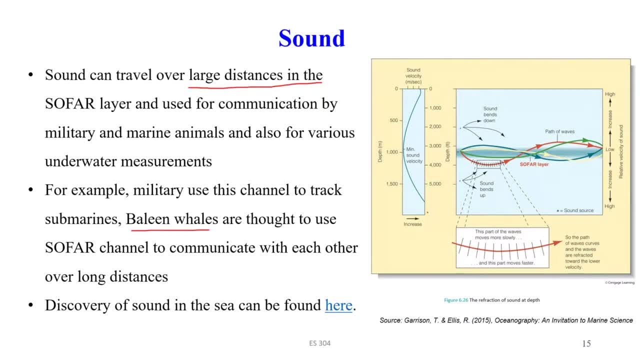 boolean whales. they are thought to use this uh channel to communicate each other. so, uh, yeah, next i'll explain the sound fixing and arranging. so, uh, yeah, next i'll explain the sound fixing and arranging. so, uh, yeah, next i'll explain the sound fixing and arranging. um, there you go. so that's the sound going. so i'm going to explain why, in the 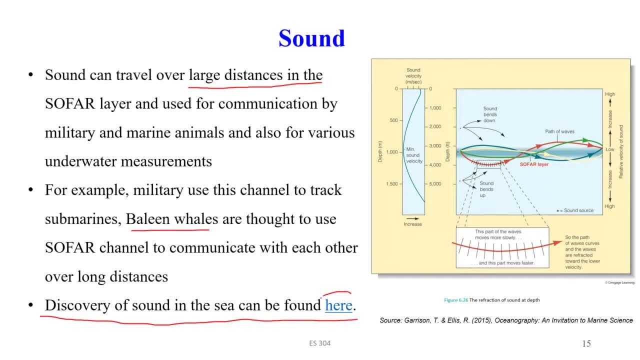 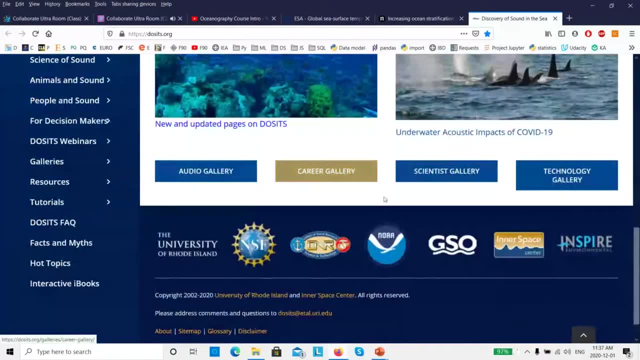 next slide. so here i just wanted to uh point out here, so i found a really nice uh the website that uh found uh that, um, you know, different uh, uh sound in the ocean, so you can, uh you can see here. so here, different gallery, so let's uh just click audio gallery here. 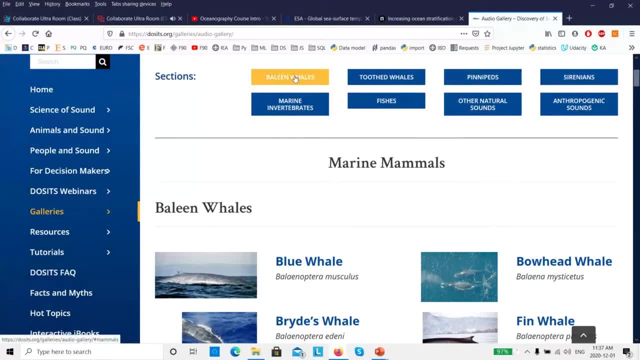 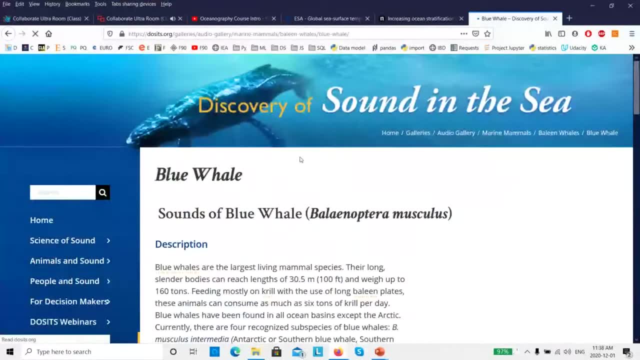 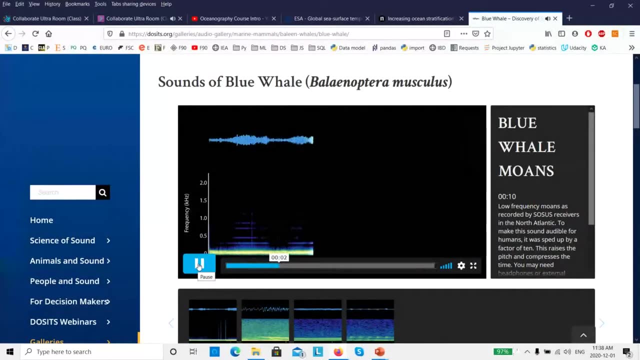 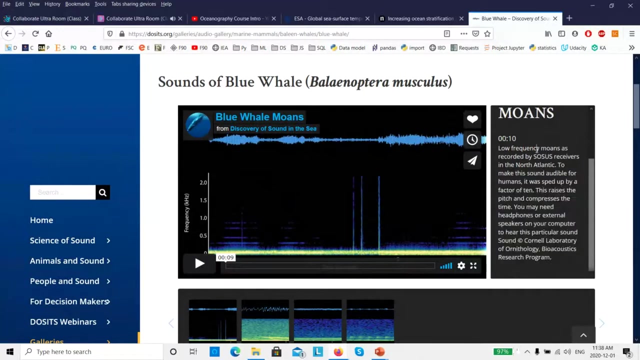 you know different marine life more. let's say that this well, and if I click here, here is the sound. so it's oh, it's quite, quite fascinating. you can have a look and also they, you know, like explanation here. so I found this is quite interesting. so what? 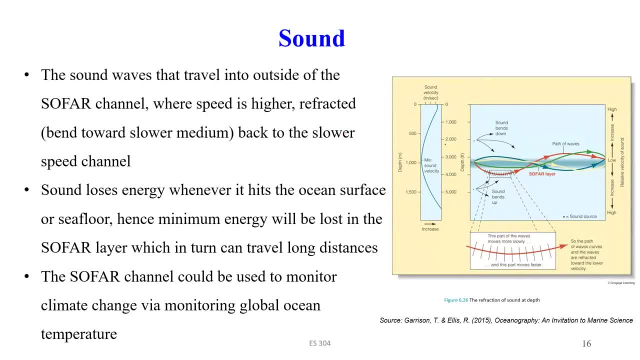 happens when the sound travels outside of the so far channel, and why it is, you know, travel long distance in this so far channel is this is because of the refraction of the sound. so what happens when the sound, you know, refracted. so it's a basic science here. 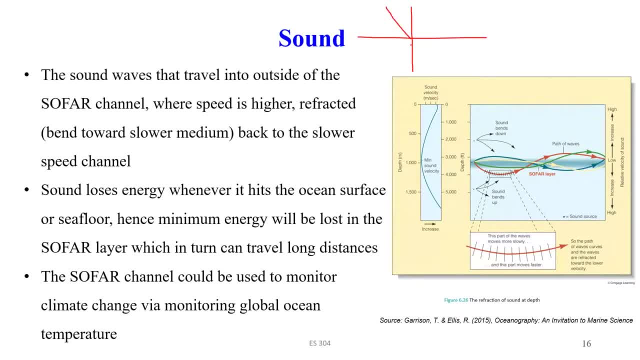 but let's draw a diagram here. so this is the incident sound. let's say the incident sound here and this is high, high sound here and this is low sound. so this incident sound when it travels, then it bent towards the- you know- lower sides, towards, you know this. 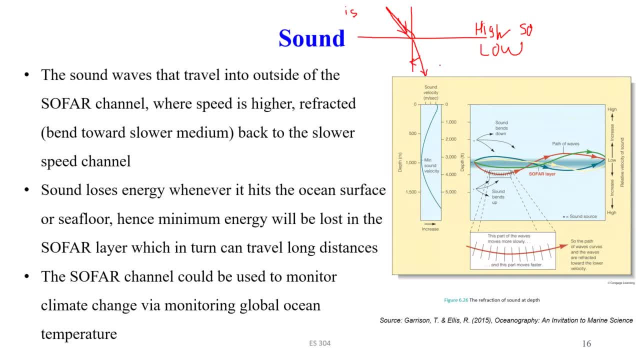 side. so this is the refracted sound, so this mechanism works here. so when in this channel, in this so far channel, this light, when the sound, sorry the sound, when it travels it, you to the fine, you know the faster speed, other, you know the channel, because this is a, this is a. 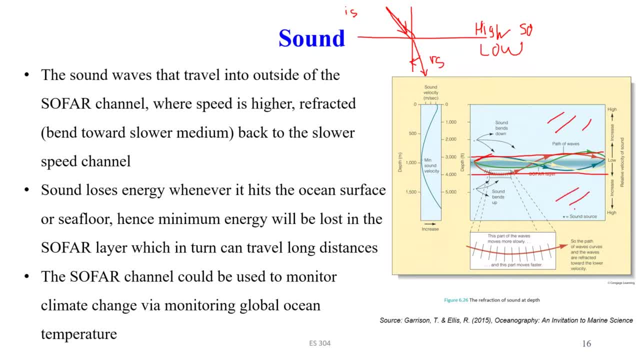 the faster outside of this so far channel they are. the speed of sound is faster here and they bent towards this back to this so far channel. so here the zoom, the, here, this, here this part of the, the waves moves more slowly. so this is the so far channel: move slowly and out of that channel this part moves faster. 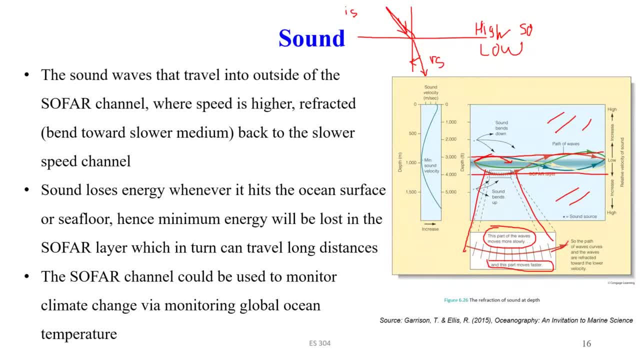 and that you know, uh, the mechanism of the bend, uh that speed of, you know, the wave, the sound, the wave of sound towards this, um, the so far channel, and where speed is higher, the refracted, that means bend towards the slower medium, back, you know, back to the slower speed channel. and sound lose energy when they encounter the. 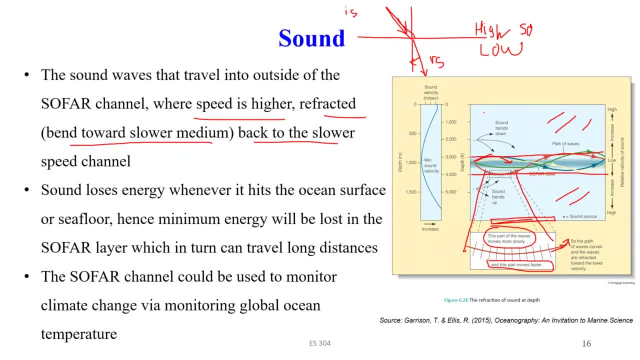 surface of the ocean, the depth of the ocean or the surface of the ocean. when they encounter bottom of bottom of the ocean and the surface of the ocean, they encounter different uh, uh, you know the particles, uh, um, the rough surface. basically, the surface at the bottom of the ocean and the surface of the ocean is, you know, the rough, because 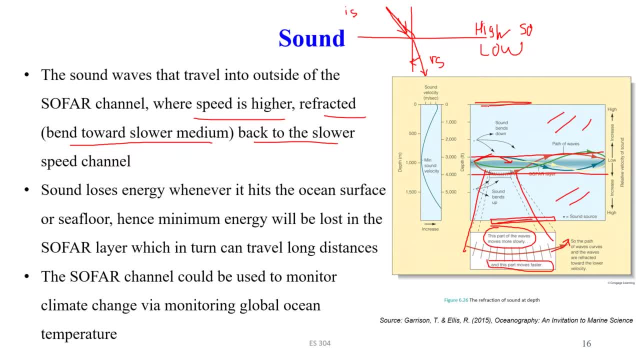 you know, rough surface because of uh different uh uh particles and uh itself are the rocks and other sediments at the bottom. they, when the sound um interact, that rough surface, they, you know scattered uh in different direction and they lose their energy. so they, that's how they lose um uh, the sound and uh in the so far channel, um uh that. 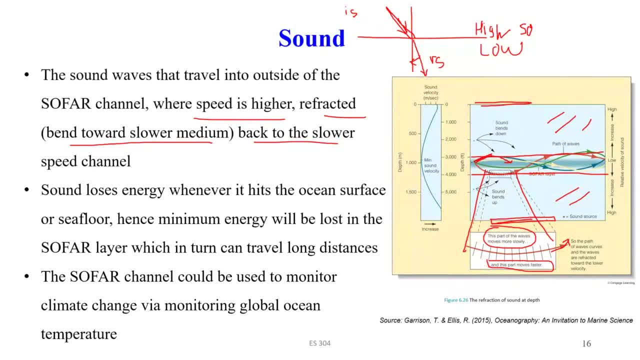 won't happen. they, they the uh the wave, sound wave. they they won't interact with uh the bottom and surface of uh the ocean and they they won't lose um the energy. so, consequently, they can travel the long distance. okay, and this technology, this uh, using this science, this mechanism, the scientists can 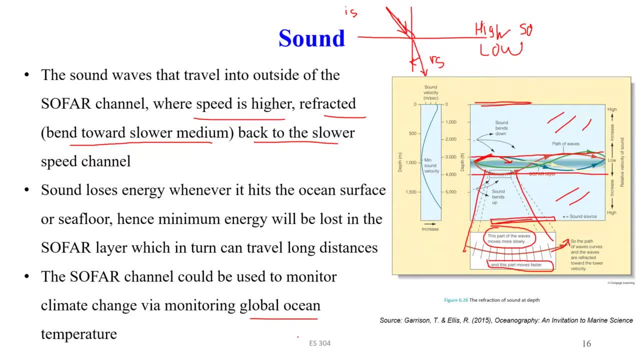 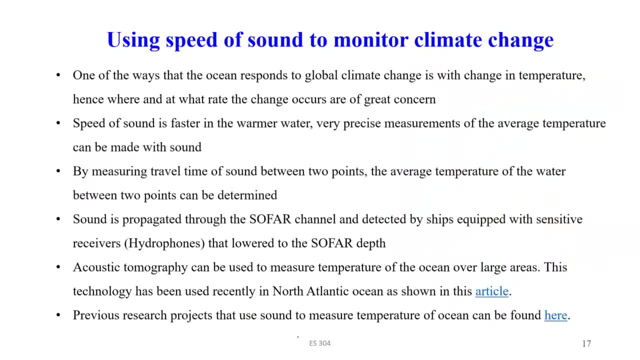 monitor the global, the ocean temperature and which is helpful to understand the climate change. so the how the scientists are uh using this um uh the sun, you know the methodology to monitor uh the climate change. so we know the temperature is one of the indicators to monitor the climate. 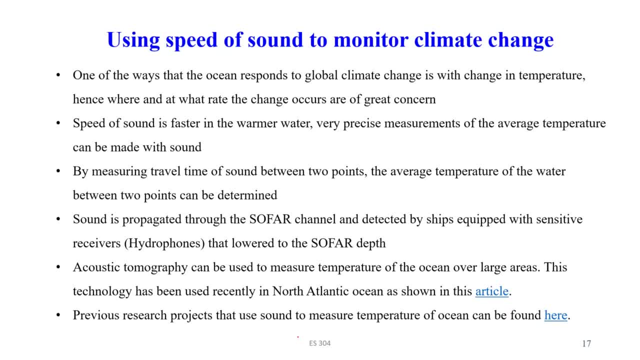 change and scientists are, um, trying to identify what is, uh, the rate that ocean is, you know warming, and where exactly that's that, uh, you know warming is happening. So scientists are trying to figure out this change with the help of this sound. So we know the sound moves faster in the warmer water and we can precisely measure, you know. 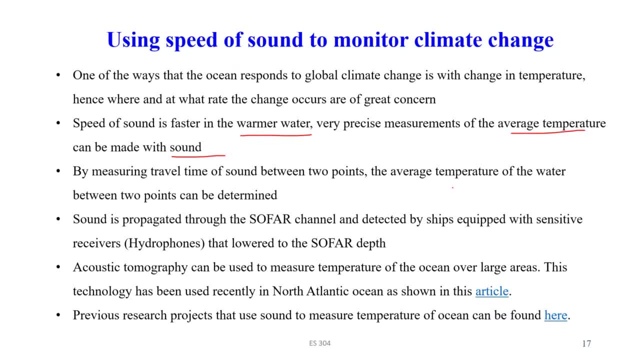 the temperature, using that the speed of sound, And we use two or many different points. Let's say an example here, the two points by you know we can measure the sound in two points and that tells you the average of you know the difference between two points. 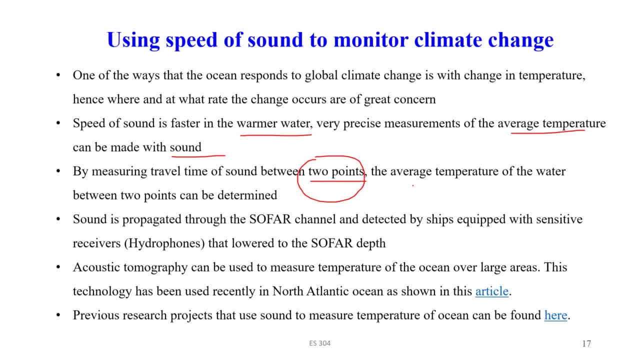 the sound, the speed of sound difference between two points tells you, you know, the temperature between those two points. so the temperature of the water between two points, okay, And sound is, you know, propagated through that so far channel and detected by the sheets. 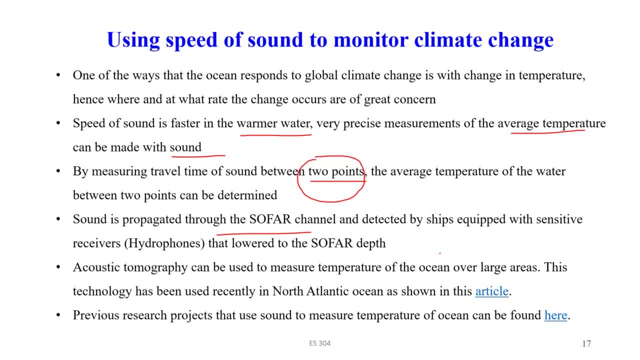 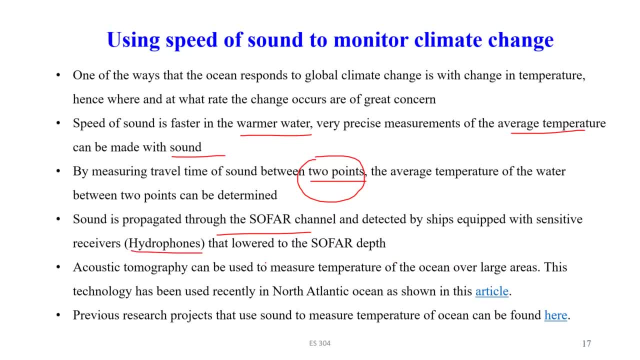 the receivers, which is called hydrophones, and that hydrophone, you know, are lower, are lowered at that that so far layer, and they can detect that the sound, and we can quantify the temperature change. And also there is another methodology, the acoustic tomography, that we can use to measure 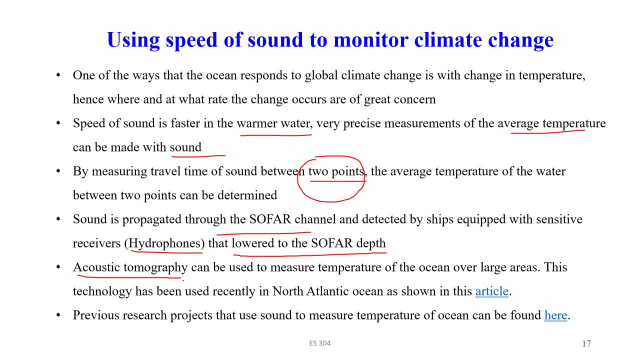 the temperature of the ocean over the large area. and this technology, you know, has been used in the past. So I have an article here you can, you can double check with this article. I hope it's not like before. So let's let's see. 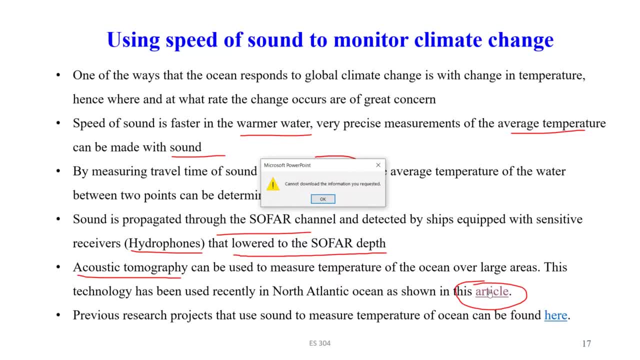 Let's click. I'm not sure what. what's wrong with this? okay? So I'm sorry about this, but I'll definitely upload. And here is a previous research project: They use the sound to measure the temperature in the ocean. okay, 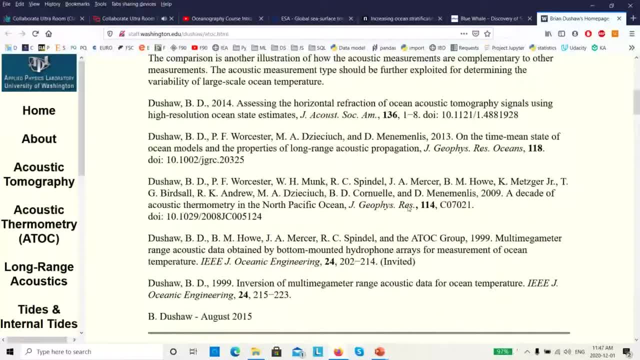 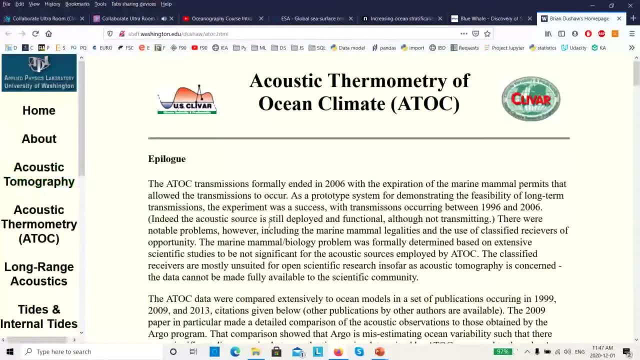 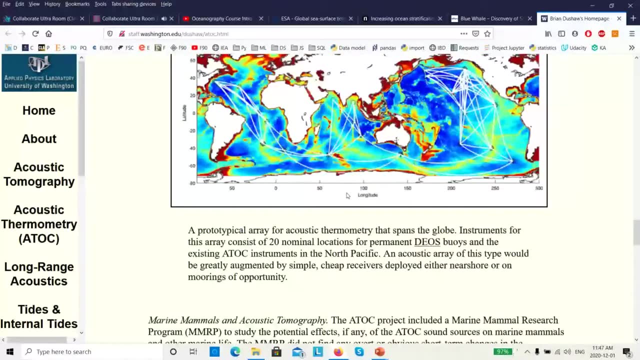 Okay, so it shows here. So there are the different projects. so here also says the: they use acoustic tomography and you know different. I mean basically there's different projects. So you can, you can go through this. at least the link worked here. 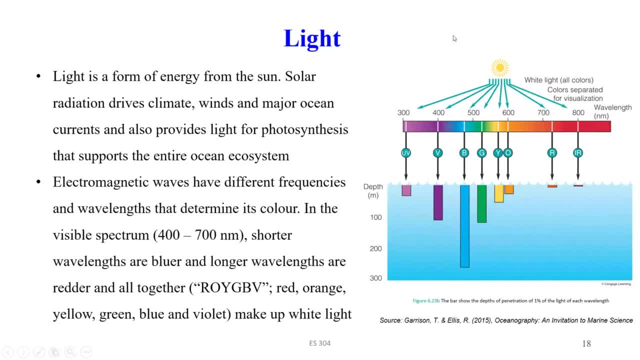 Light is another form of energy, And the solar radiation, Yeah Yeah. So the energy from the Earth is. the ocean receives maximum solar radiation And you know that radiation provides the lights for photosynthesis. Without the photosynthesis process, it's life is impossible, almost impossible in the 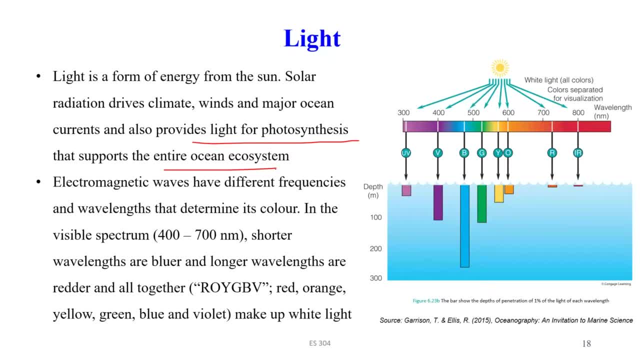 you know entire ocean ecosystem and also that the surface layer, the energy receiving the surface of the ocean, drives the climate and you know different patterns of the winds. and the energy we receive from sun is a form of electromagnetic radiation and the electromagnetic waves have different wavelength and frequencies. that determines 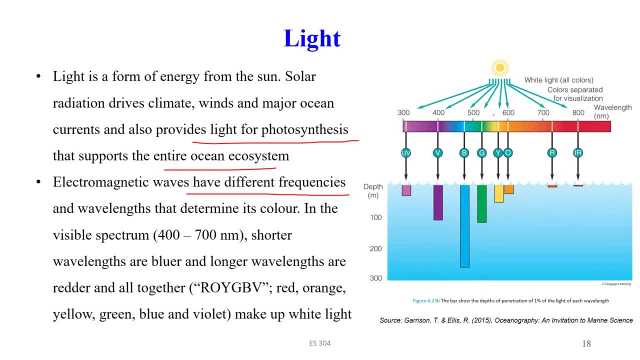 the color of the radiation, so in the visible spectrum which we can see here. so which is the wavelength from 400 nanometer to the 700 nanometer. so this is a visible- we call visible- range of the light and shorter wavelengths are, you know, towards the blue here. 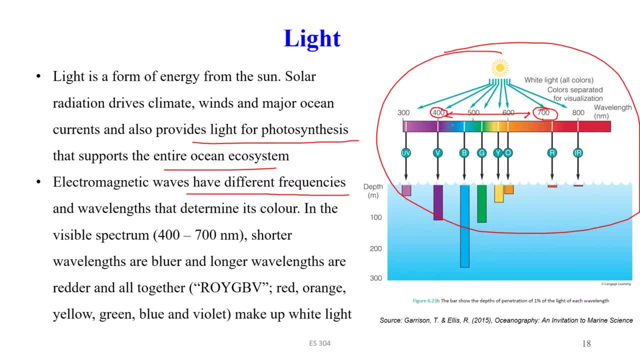 so it 400. it's a kind of the purple, but you know it's the towards the blue region and when we go, you know the long wave radiation it kind of you know it's towards the red. okay, so here, red, orange, yellow, green, blue and the violet color. so this is basically the color. 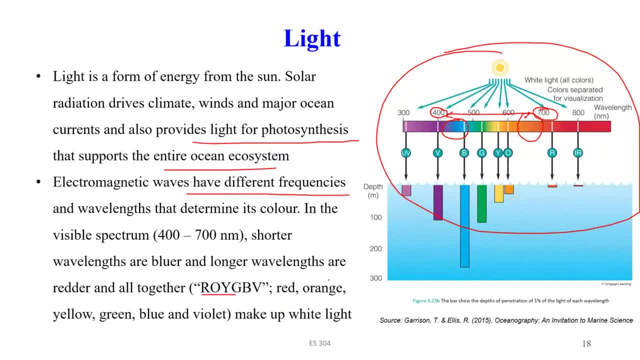 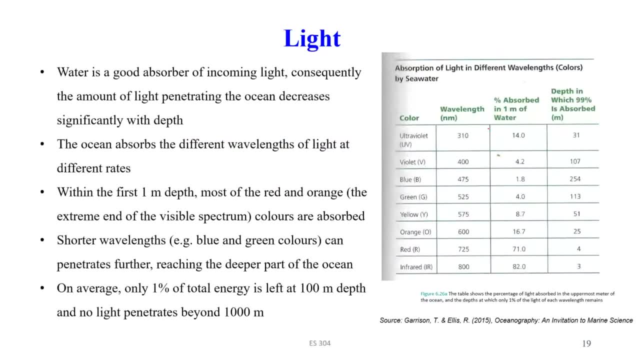 which is not the color of the light. so for the single silver particles in the uh observe the light in different rate, okay, And consequently the penetration of light in the ocean is different based on their- you know- wavelength, Here the UV radiation. 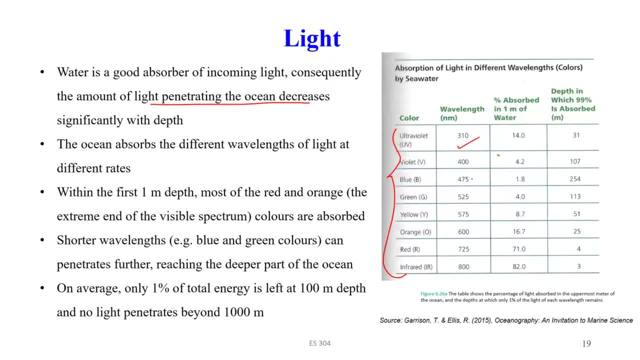 which is the wavelength is 310.. It's obviously out of the visible range And this column here shows percentage absorbed of, you know, the radiation in one meter of the water depth. So basically here what is the percentage of, you know, absorption, So the UV radiation. 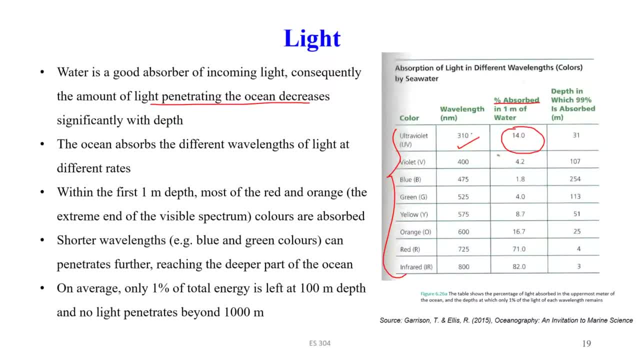 absorbs 14% of radiation per meter, 14% of UV radiation at one meter within the one meter depth of the water, And similarly, you know there are other number we can see here in this column And looking at this column, 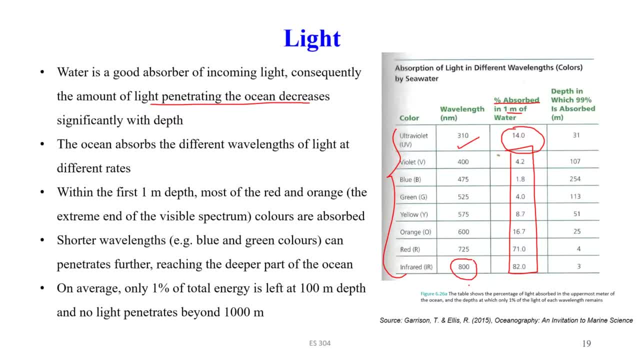 the infrared, which is higher in, you know, wavelength, the 800 nanometer in the wavelength that is absorbed, 82% of that infrared radiation absorbed within the water depth of the water. So within one meter you know depth of the ocean water. okay, And as we discuss here, 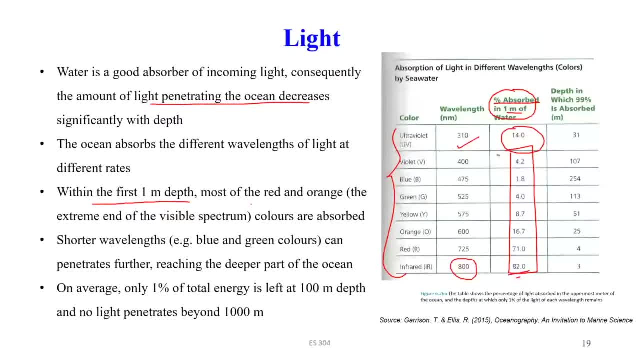 on the table. so within first one meter most of the red and orange colors are absorbed. So basically, that is, you know, extreme end of the visible spectrum. So here you know red and the orange. they are the, you know longer, the wavelength, and these are absorbed. 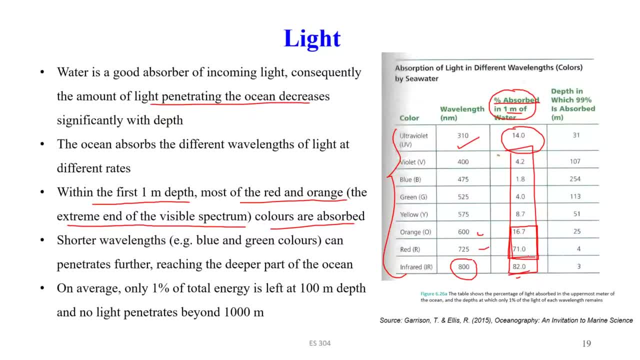 mostly in the surface layer, so within the one meter of the ocean layer, And only the blue, green colors they can penetrate. you know, the deeper layer- It's not we said a deeper layer, you know deeper than this layer, that one below than the one meter, basically. And 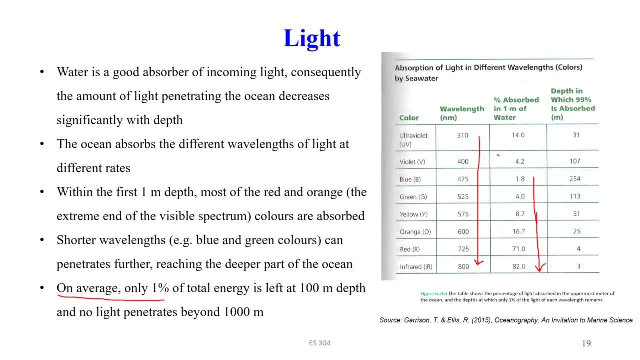 on average, only 1% of total light energy is, you know, available at 100 meter depth. So, basically, if we look at the last column here, which is the absorption in, you know the depth, it shows that it's a bit, sometimes bit confusing, but it's the depth, The depth. 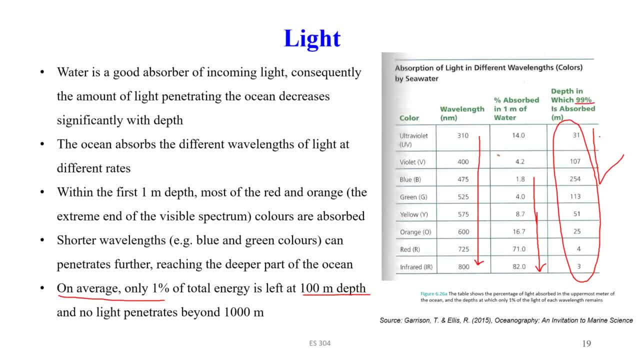 is in meter where the light is coming from. So it's the depth where 99% of the energy is absorbed within that depth. For example, the ultraviolet, the radiation, that energy is 99% absorbed within 31 meter depth of the. 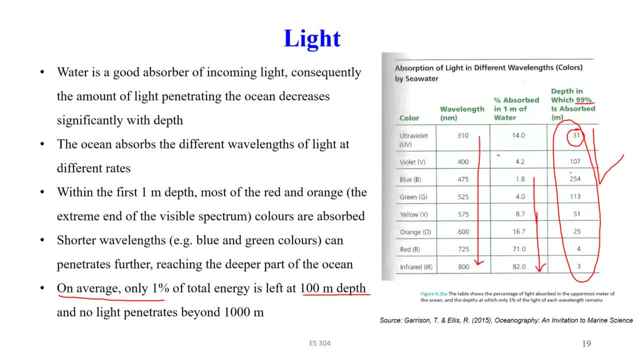 water, the ocean. Okay, So the blue light which can, which is the deepest, can go that in a blue light. So the blue light can reach 254 meter. 99% of the blue light can reach 254 meter. So 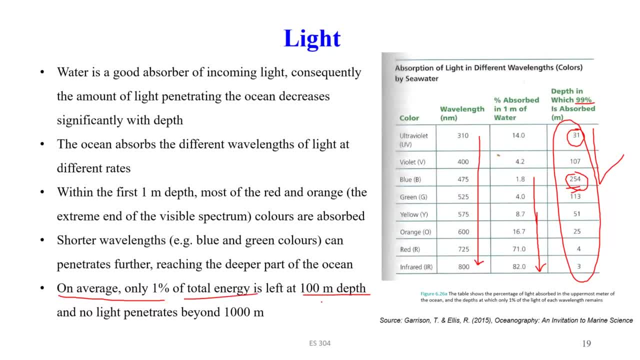 here the 1% of total energy is left, 100 meter depth. So that must be, you know, blue and the green, because it can grow deeper than the other, the radiation, And also the blue, the green, that's the blue light. So the blue light can reach 254 meter. So here, 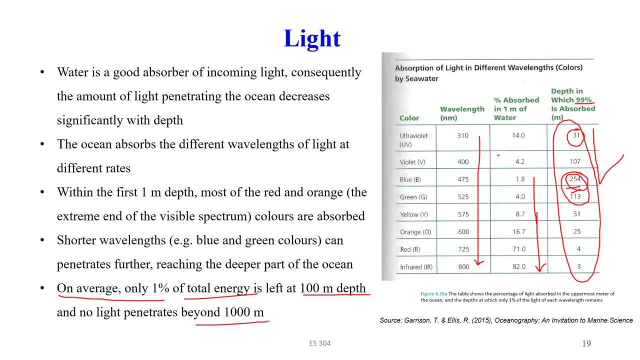 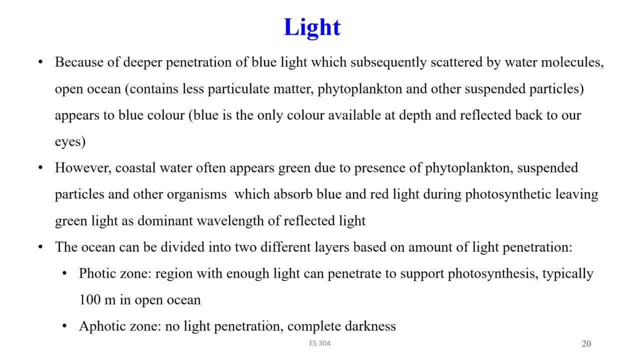 the blue light can reach 254 meter. So here the 1% of total energy is left 100 meter depth, and beyond 1000 meter there would be no any light penetration. okay, so the deeper penetration of some blue light, which is, you know, we can see blue because they. 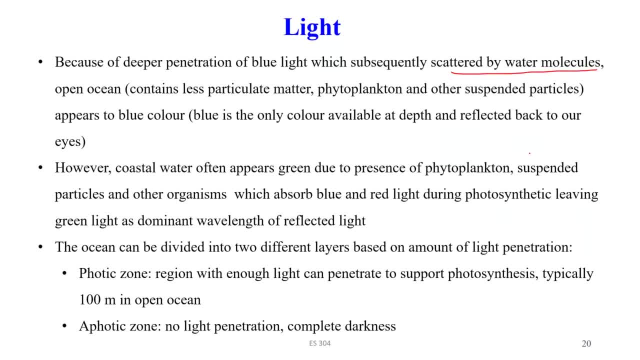 are scattered by the water molecules, we can see the blue light because water molecules scattered the blue light in in open ocean- mainly we can. there would be no particulate matter or phytoplankton and other suspended particles in the clean water. open water is basically the clean water and the blue light can. 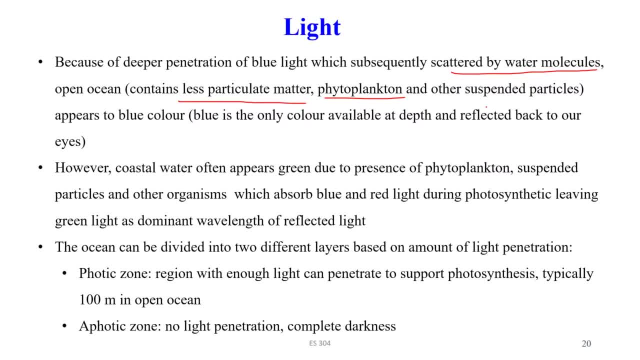 penetrate its maximum capacity and that is scattered by the water molecules and we can see blue ocean. That's why, when we look from the top, the you know ocean, the open ocean, looks, you know, blue color. Okay, But yeah, so here it's just trying and looking at here So it appears. 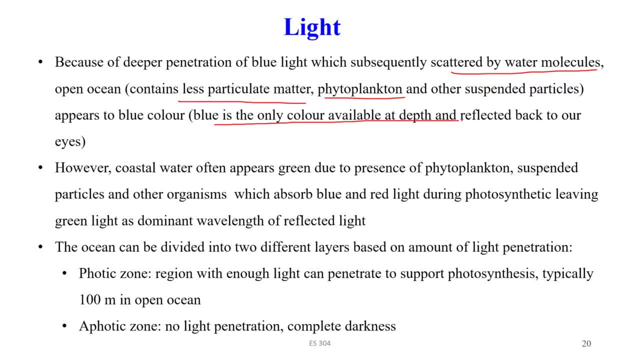 blue because blue is the only color available at that depth and reflected back to our eye. So that's why we see the blue color. But in the crystal region we have different, you know, like pollution, pollutants, in terms of, you know, there are many plants, the phytoplankton. 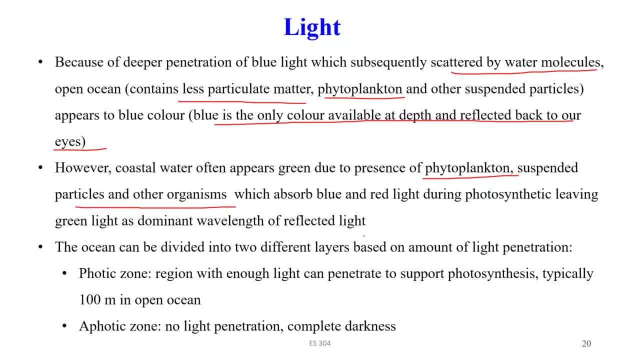 suspended particles and other different organisms. They absorb blue light and also the red light during their the processes, the photosynthesis process, And only they leave the green light and that is the dominant wavelength of light, the green light in that coastal region, and we see that, you know, reason is the green color and 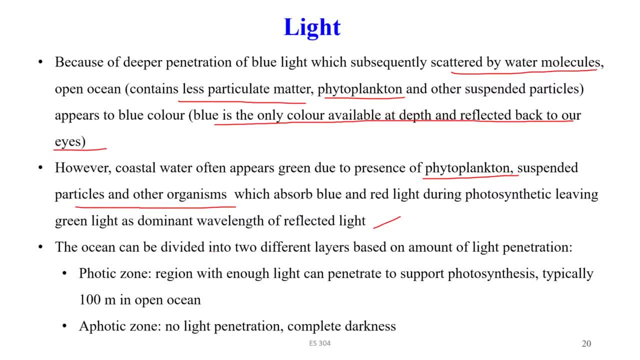 based on that absorption of the light, we can divide ocean into two different layers. So now one is the photic zone and other is a photic zone. so the photic zone basically the reason of the enough light, you know, that can penetrate to support the photosynthesis process and basically it's the ocean, you know, like a top.